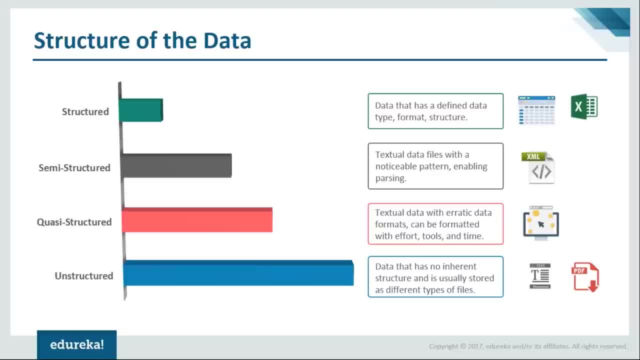 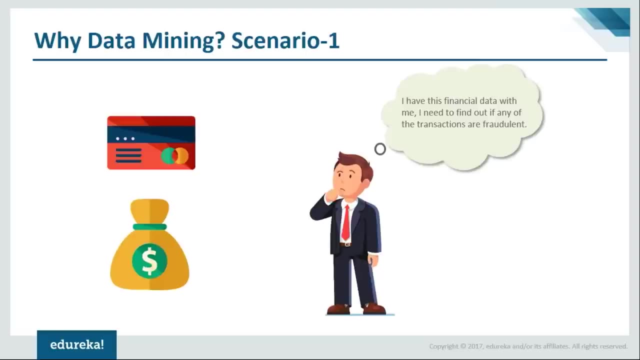 But with a bit of tweaking, information can be extracted from it. Unstructured data has no inherent data format at all, And that is why extracting information from it can be quite a cumbersome task. You've understood that data comes from multiple sources and it is also available in. 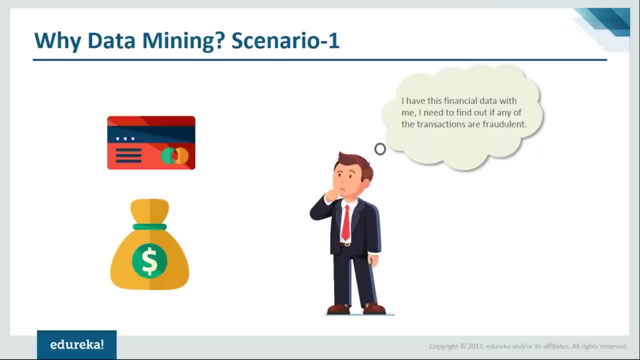 different formats. Now let's see what can be done with the data which we have with us. This is John, and he comes across financial data And he's trying to understand how many of these financial transactions are fraudulent. Now John stumbles upon the email data and he's trying to figure. 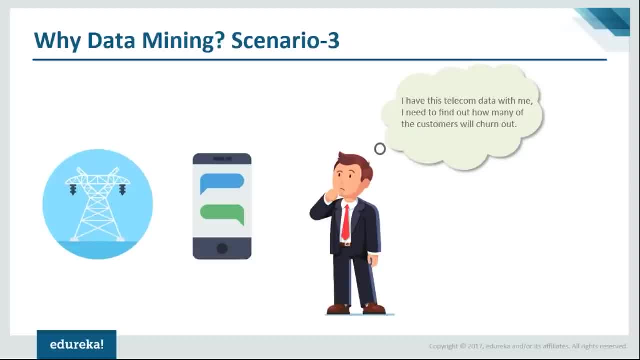 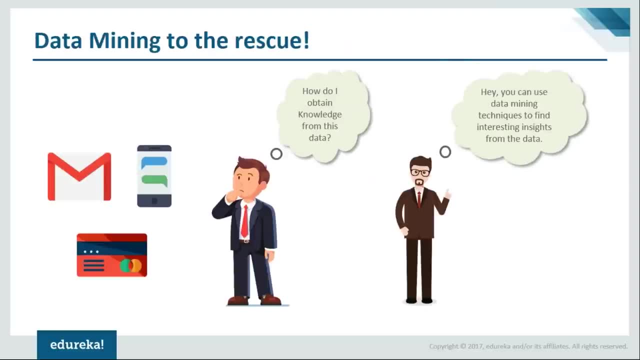 out how many of the mails are spam. John notices telecom data and he wants to find out how many of the customers will churn out. John does have the data with him. How does he obtain information from it? So his friend Jim is a data scientist. 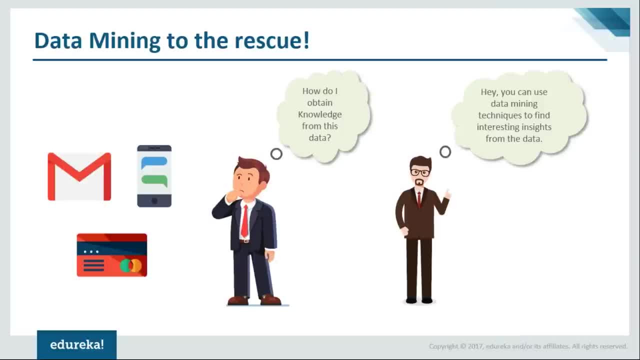 Who suggests him to use data mining techniques to find solutions to each of the three problem statements. That is, John can use data mining techniques to find out how many of the financial transactions were fraudulent. Similarly, he can also use data mining techniques to find out if 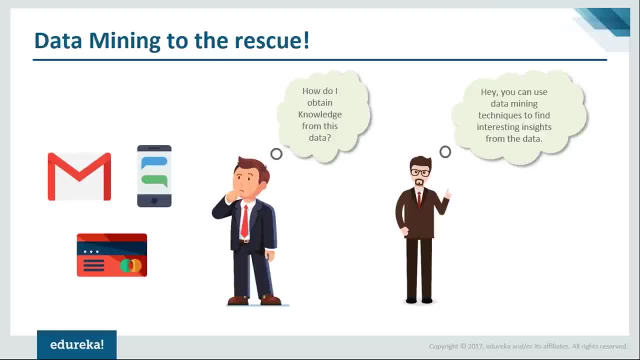 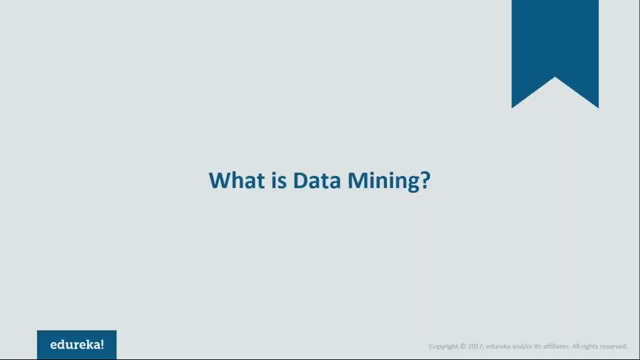 the mail was spam or not. And again, John can again use data mining techniques to find out how many of the customers will churn out If understood the need of data mining. now let's understand what the data mining techniques are. So let's see what the data mining techniques are. So let's 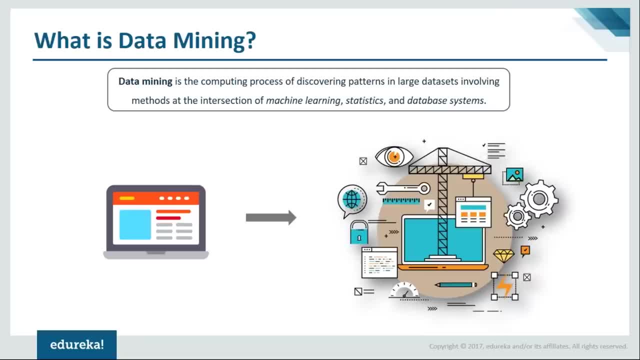 see what exactly is data mining. Let's look at the definition. Data mining is the computing process of discovering patterns in large data sets, involving methods at the intersection of machine learning, statistics and database systems. Now, that is quite a complicated definition. So what do? 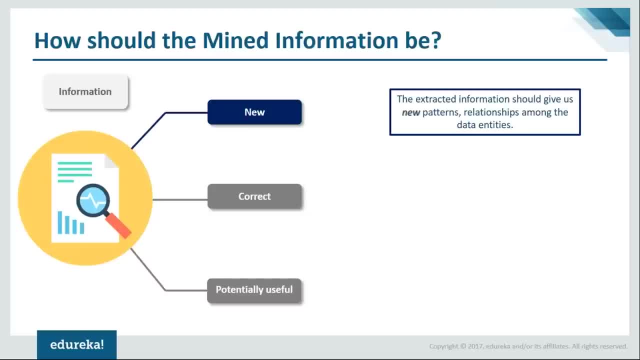 we exactly mean by that? In simple terms, data mining is mining of information from data which is new, correct and potentially useful. Now let's understand. why should the mind information be new? Let's take an example. We have a data set. 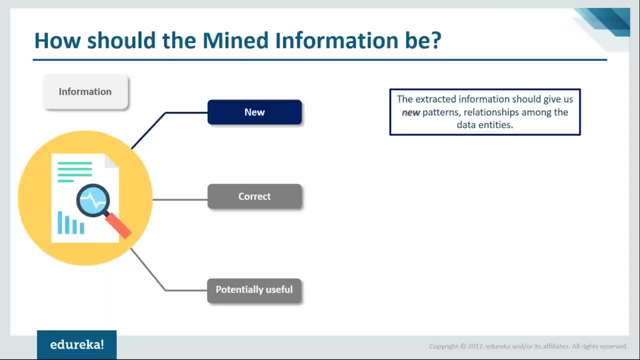 with us. We apply some data mining techniques, find out a pattern, and this pattern tells us that smoking causes cancer. Now, this is not something new. We already know this. We've invested time, we've invested effort and we've found out information which we already know. So it doesn't. 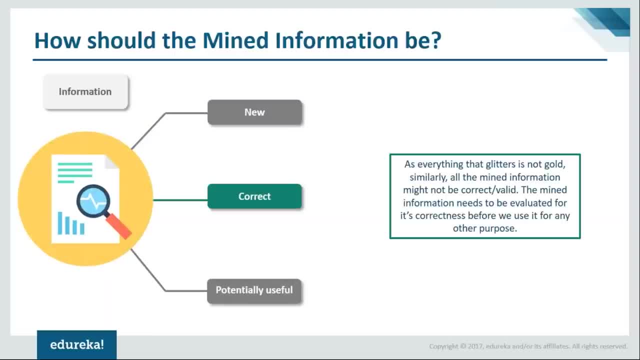 really serve a purpose. Let's look at the next parameter. the correct answer. The correct answer is the correctness of the information. Let's again take an example. We have a data set which comprises of the stock prices of all the companies, And we predict that a company X its stock price. 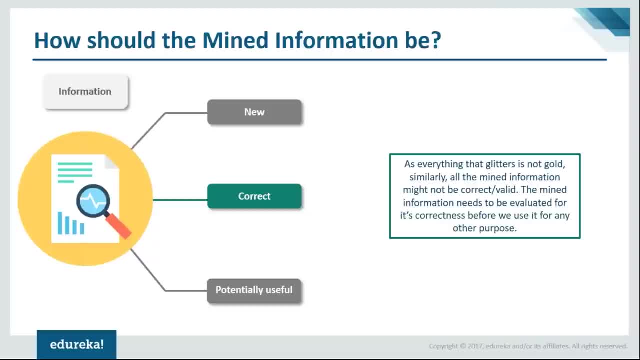 will increase by 20 percent in the next week, But, on the contrary, what actually happens is its stock price decreases by 10 percent. What happened over here? We found out information which eventually proved to be wrong, And that is why we're going to look at the next parameter, the correct answer. 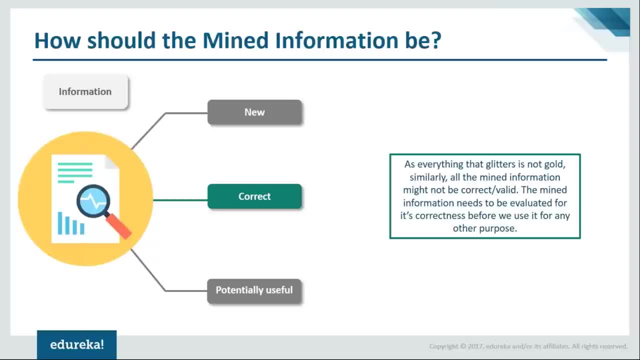 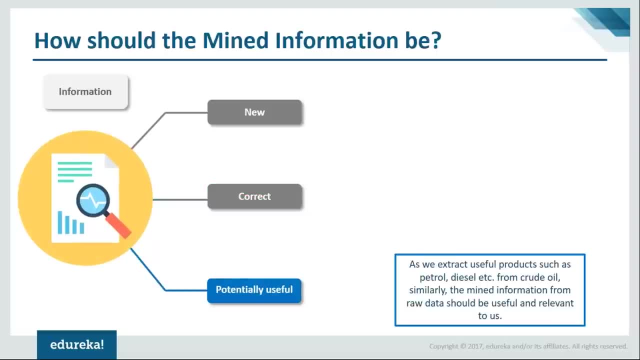 And that is why it is always necessary to check the validity of the information before we reach to any sort of conclusion. You understood that the information is new and correct. Now it's time to see if the information is useful or not. As we saw in the first example, we found out an information. 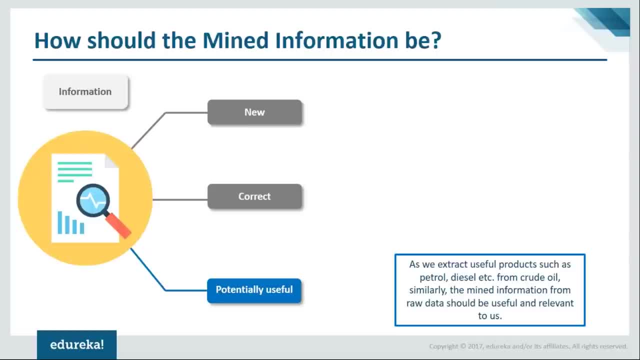 which told us that smoking causes cancer. Now, that information did not serve a purpose, So, instead of finding that information, what we can do is we can find out patterns which would tell us the longevity of a person who smokes and the longevity of a person who does not smoke. 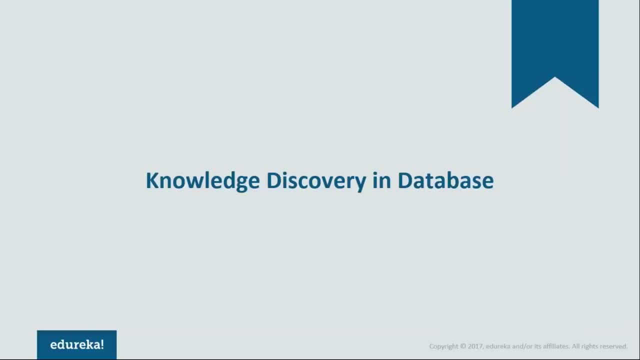 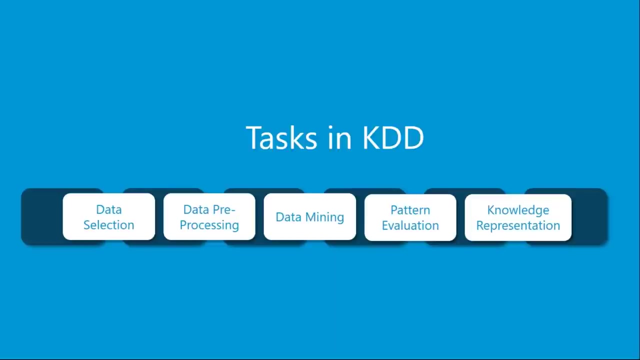 This information will be more useful to us. You've understood what is data mining. Now let's look at the sequential steps in discovering knowledge from the data. KDD has these steps: Selection of data, pre-processing of data, mining of data, evaluation of patterns and representation of knowledge. 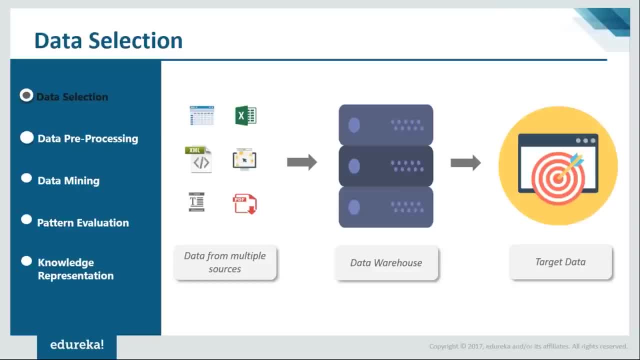 Let's start with the first step, which is selection of data. We already know that data comes from multiple sources and that is also available in multiple formats, So our first task would be to integrate all of this data and store it in one single location, which is the data warehouse. 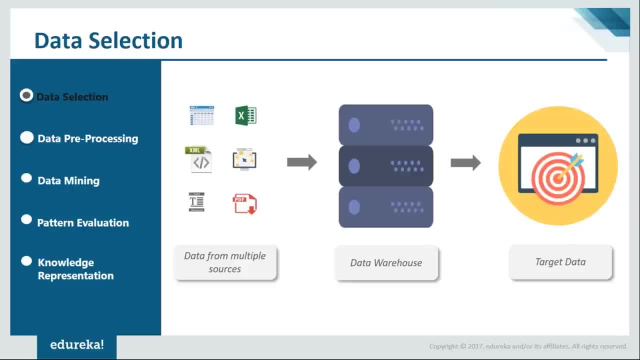 So we've integrated the data, stored it into a data warehouse. Now we can select one particular data set on which we would want to do our analytical task. The data selection has been done. Now it's time to do some pre-processing, Pre-processing tasks. 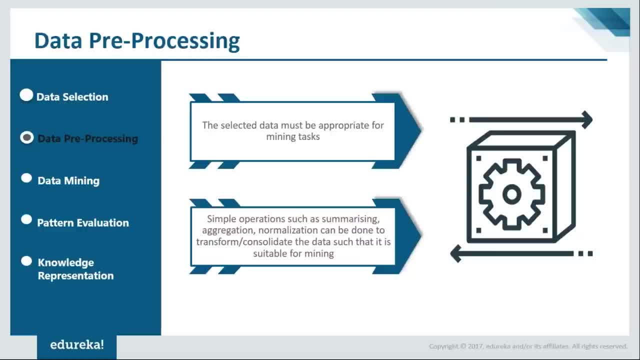 involve, such as understanding the structure of data. We can also use visualization techniques to understand how are the variables in the data set related to each other, the correlation among them. You can also apply simple operations such as summarizing, aggregation and normalization. Data selection has been done. We've also done a bit of pre-processing. 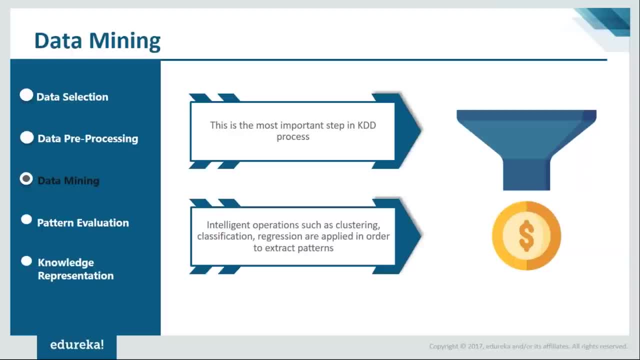 Now it's time for the most important step in dolphins process, which is mining data. You already know what does data mining. Let's understand how can we do it. So theta mining is applying of intelligent operations such as clustering, classification, regression and so on. We apply these intelligent operations and extract. 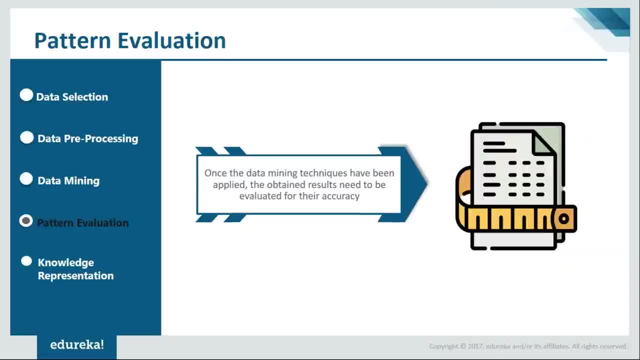 by tools. So, when it's applied, intelligent populations with opt-in patterns. Now it's time we check for the validating thought to be the pattern. Now it's time to check for the validating of these patterns. That is, we do the three parameter check. We need to see if 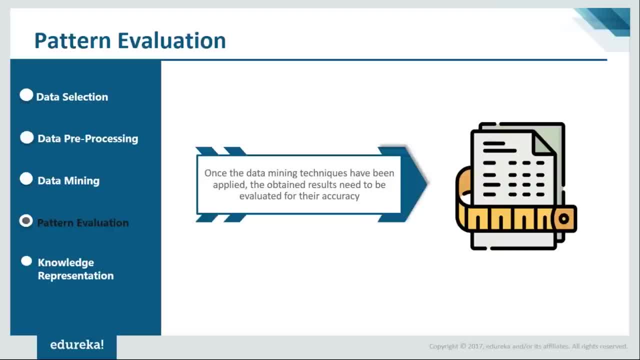 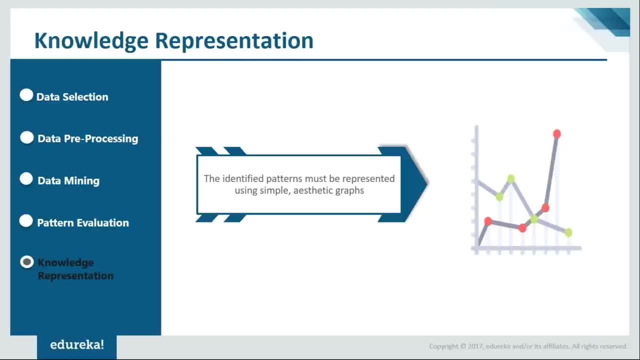 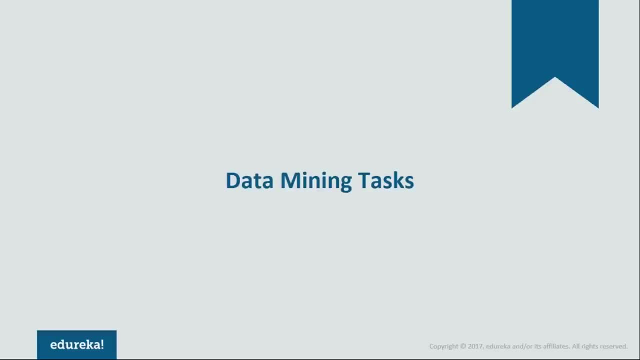 the obtained information is correct, useful and new. Once the information is validated, now it's time to finally represent the information using simple and aesthetic graphs. Those were the sequential steps involved in KDD process. Now let's look at the data mining techniques. In this session, we'll 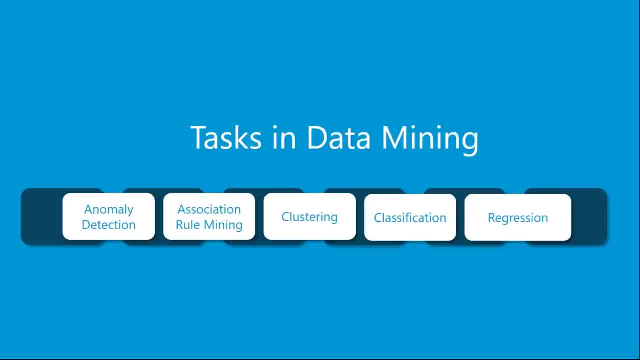 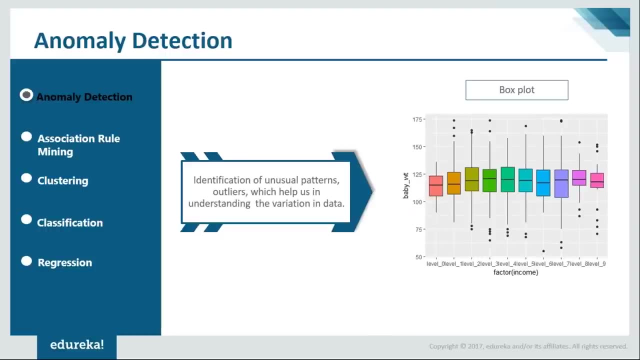 be looking at anomaly detection, association rule mining, clustering, classification and regression. Let's proceed with the first data mining technique, which is anomaly detection. This technique helps us to identify unusual patterns or outliers in the data. Let's take an example. There's a movie. 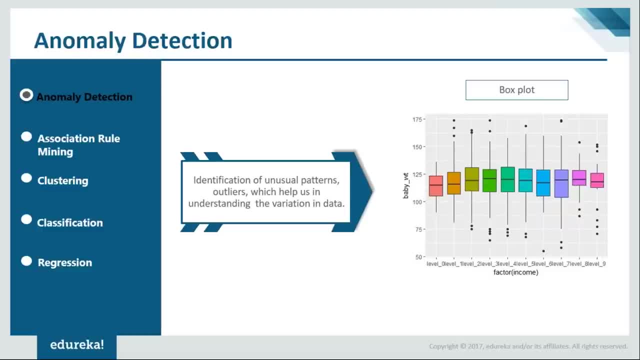 theater, and the average salary of people who go to watch a movie in that theater is around rupees fifty thousand per month. One fine day, it just happens that Mr Mukesh Ambani decides to watch a movie in this theater. So what happens? The average salary shoots up and it shoots up. 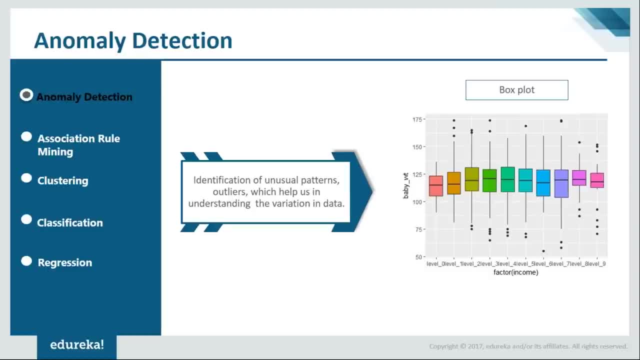 sky-high. So in this case, Mr Mukesh Ambani would be the outlier or the anomaly Prior to processing of the data. we need to make sure that we do some processing on the outliers. That is, either we remove the outliers or we do a. 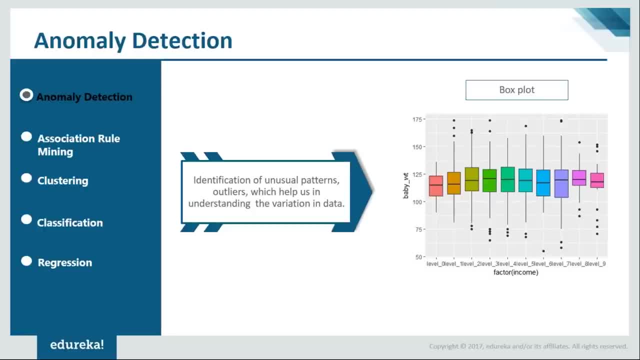 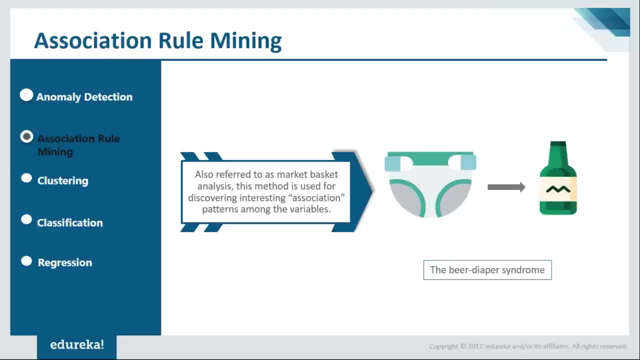 bit of adjustment to the outliers, And then we come to the main analysis part with the data. The next technique is association rule mining. This is also known as market basket analysis. This has a very interesting example and it goes by the name of the Biodipo syndrome. So 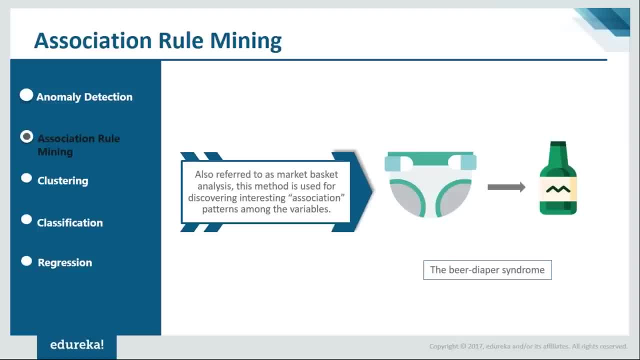 in a survey done by a supermarket, it was found out that whenever a single father came to the store to buy a diaper, there was very high likelihood that he would also buy a bottle of Biodipo. Now that's quite an uncanny relationship, isn't it? A single father coming to a 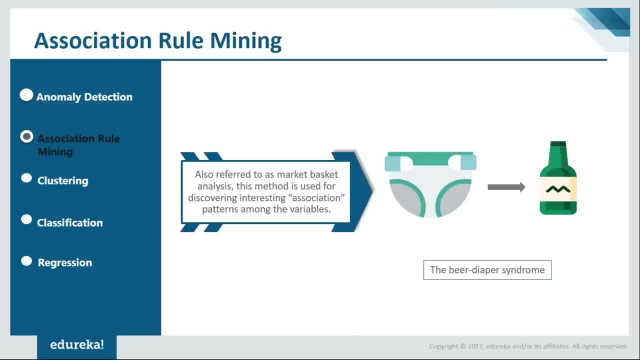 store to buy a diaper also buys a bottle of Biodipo. Quite strange, But this is what the supermarket was able to find out with the help of association rule mining, And this is also the basis for many of the recommender system. Let's take 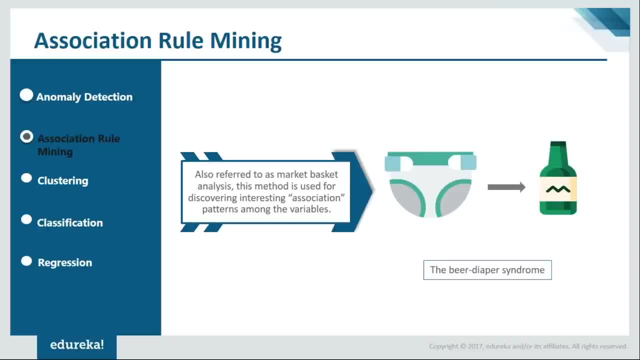 Netflix. Suppose you watch the TV show Friends on Netflix, The recommender system also suggests you to watch How I Met Your Mother and Big Bang Theory. Why? The recommender system understands that all of these 3 TV shows belong to the Comedy genre And therefore, if you watch Friends, there is also a high likelihood. 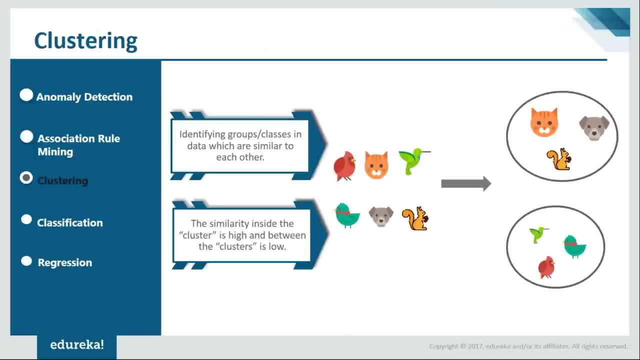 that you might watch Big Bang Theory and How I Met Your Mother. Next comes clustering. This comes under the purview of unsupervised learning. So, with the help of clustering, if you have a set of observations, we can segregate these observations into clusters on the basis of their similarity. 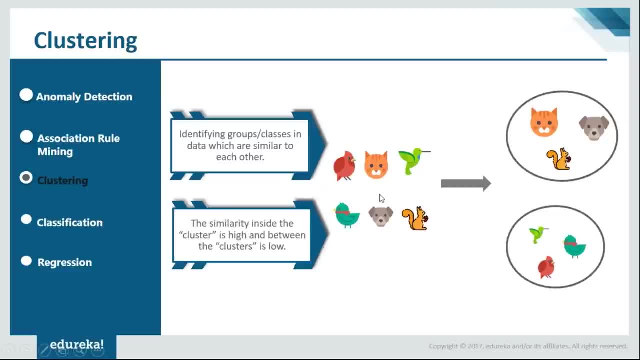 Let's have a look at this slide. We have this set of observations and we are obtaining two clusters from these. So the first cluster comprises of all the animals and the second cluster comprises of all the birds. and this clustering has been done on the similarity of the observations, that is, there is high. 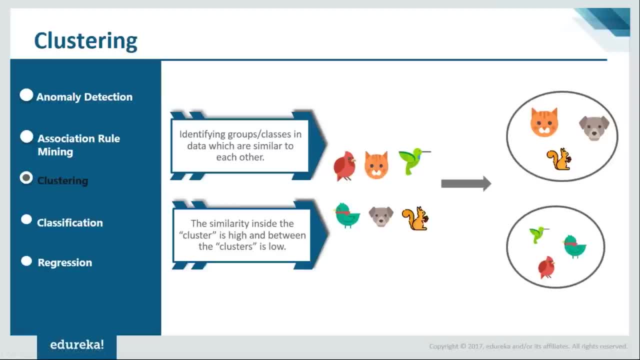 intra-cluster similarity. So what do I mean by high intra-cluster similarity? That is, all the observations in one cluster are similar to each other. so if we see over here, all of these are animals and they are similar to each other. and in the second cluster all of them are birds and they're quite. 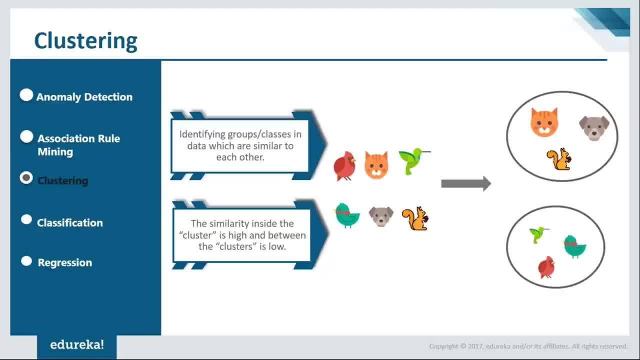 similar to each other, PSut. when we compared these two clusters, what happens is there is very low similarity or there is quite a bit of dissimilarity, and this is the basis for clustering. Now, I've said that clustering comes under the poor view of unsupervised learning. 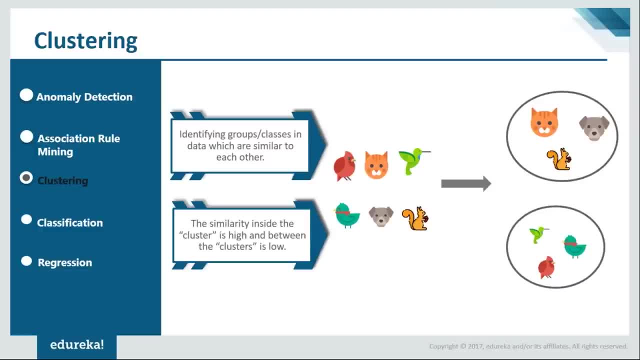 so what is unsupervised learning? Now again, unsupervised learning comes under meta-cluster, corpo-acak learning, and that is a common practice for scientists rather than maybe an argument. we are going to be more drain to more specific topic for these. So this one: What do I mean by meta-clusters? 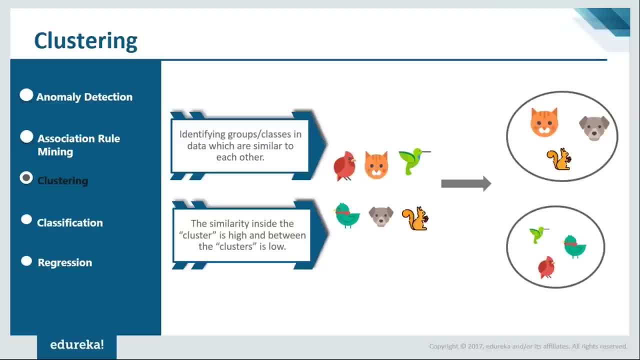 comes under the domain of machine learning, and machine learning algorithms are algorithms which learn on their own, So coming to unsupervised learning. they do not have predefined labels, So what we see over here are: we just have observations and there are no labels which. 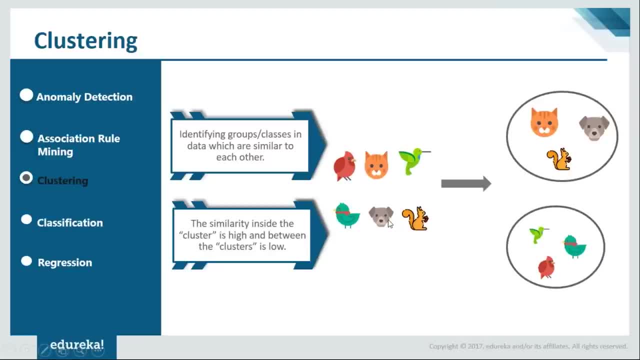 tell us that this is an animal or this is a bird, but even then, the unsupervised learning algorithm is able to cluster them, and the clustering has been done on the basis of similarities of these observations. It is only after the clustering has been done that we understand that all of the 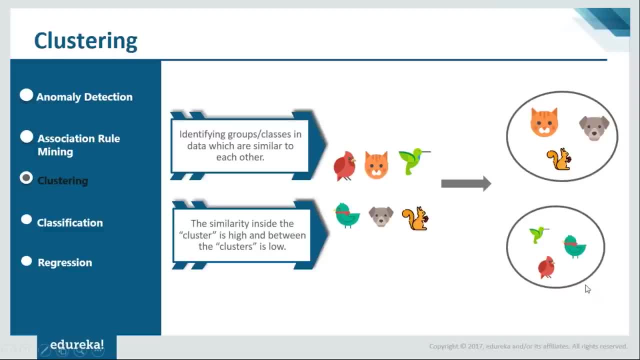 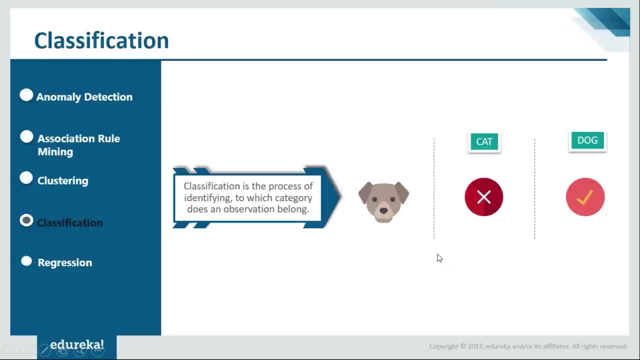 observations in the first cluster are animals and all of the observations in the second cluster are birds. The next technique is classification, and classification comes under the purview of supervised learning, and in supervised learning we do have predefined labels. So let's take a look at the slide. We have an observation and we have two labels, which are: 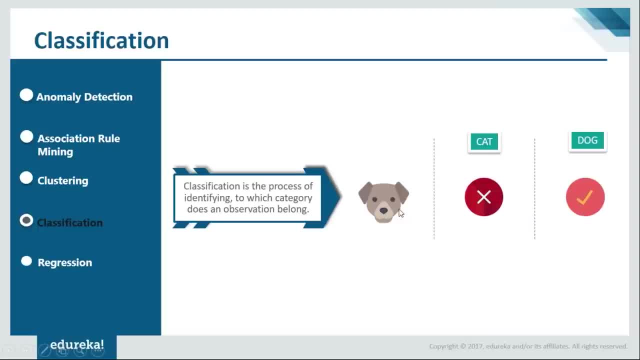 categorized Cat and dog and our task is to assign a label to it. So what are we doing over here? So what happens in classification is we have an observation and we try to classify it into one of the categories. So for this slide, if we assign the observation, the label of cat, then the classification would 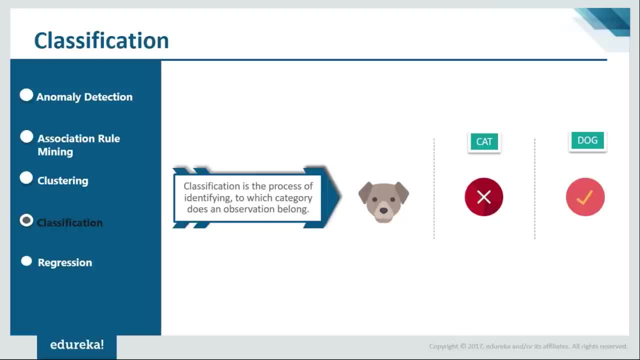 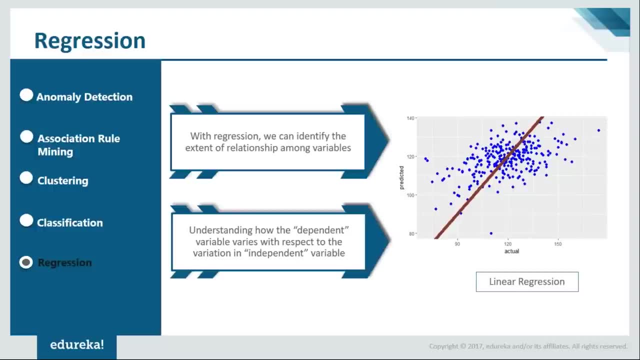 be wrong. If we assign the label of dog to it, then the classification would be right. The next technique is regression. With the help of regression we can find out how does one variable change with respect to another variable. Regression again comes under the purview of supervised learning and therefore we have labels. There are many types of 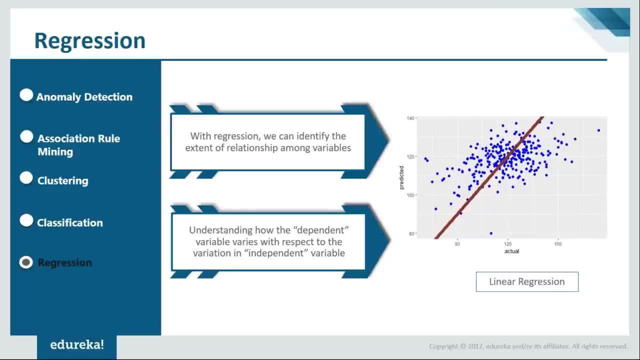 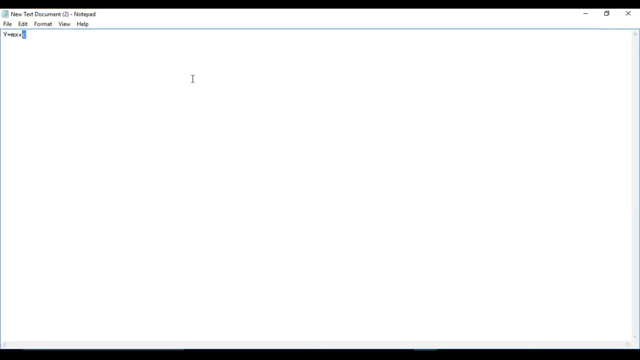 regression techniques such as linear regression, logistic regression, Poisson regression and so on. And for the sake of this session, I'll give a brief intro to linear regression. Now all of you must have come across the equation of a straight line, which is: y is equal to mx plus c. 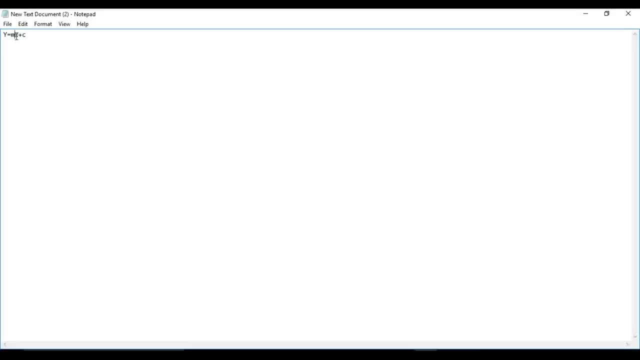 Over here. y will be the dependent variable and x will be the independent variable, and we are trying to understand how does y vary with respect to x? That is the basic idea behind regression. We have one dependent variable and we try to understand how does this dependent variable 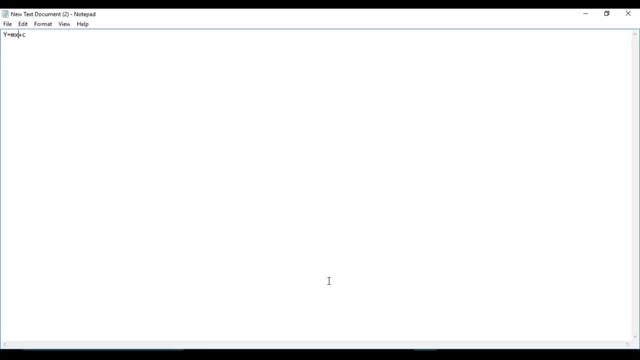 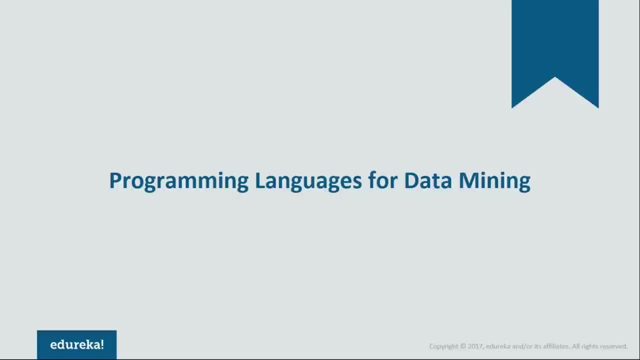 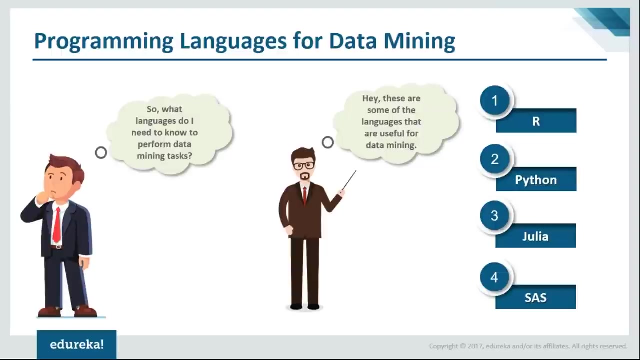 change with respect to the independent variables. We've looked at some of the most commonly used data mining techniques. Now it's time to have a look at some of the programming languages used for the purpose of data mining. We have Jim again, and Jim tells us that we can use R, Python, Julia. 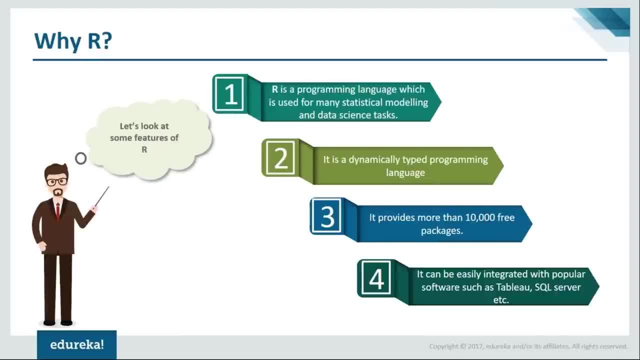 and SAS for our data mining tasks And for the hands-on. since I've used R, let's understand some of the features of R Now, why am I using R? So R is a programming language which is used for many statistical modeling and data science tasks and I believe 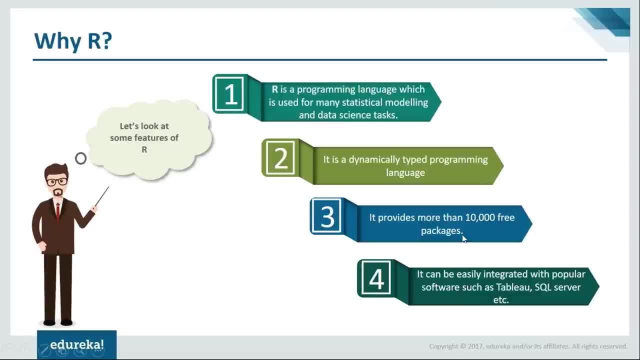 one of the best features of R is that it provides more than 10,000 free packages, Whatever your need is. if you want to do data visualization, R provides a package for that. If you want to do statistical analysis, R provides a package for that. If you want to do data, 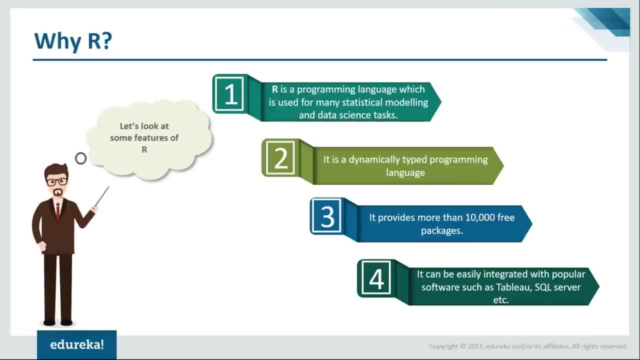 manipulation. R also provides a package for that, Isn't it great. R is also a dynamically typed programming language. What do I mean by it? So the focus is on the value of the variable and not on the data type of the variable, and because of this, we can make statements in R such as: so the first statement. 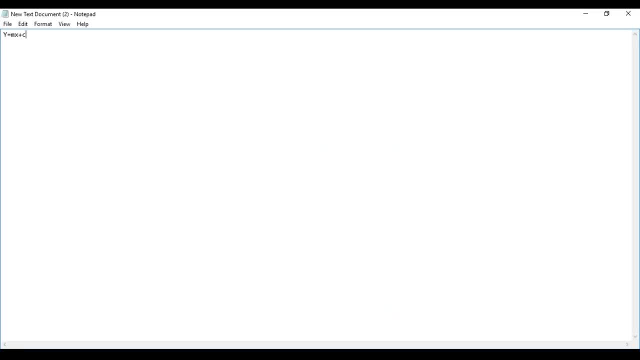 would be: a is equal to 10 and the next statement would be: a is equal to. and So we see over here that the focus is not on the data type. For the first case we are assigning an integer and for the second case we are assigning a string, and this has the basic idea of a dynamically typed programming. 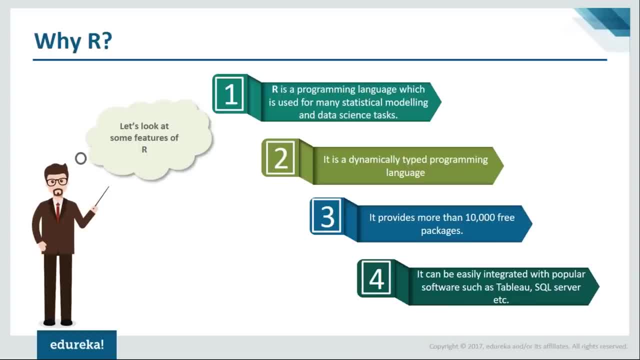 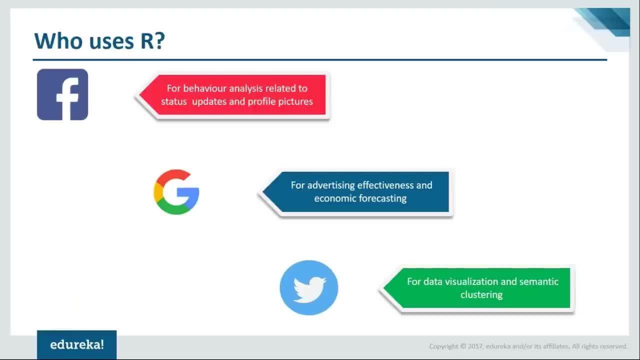 language. Another feature of R is it can be easily integrated with other popular softwares. Some of the examples are Tableau and SQL Server. You understood why R. Now let's look at who uses R. So this slide tells us that the big 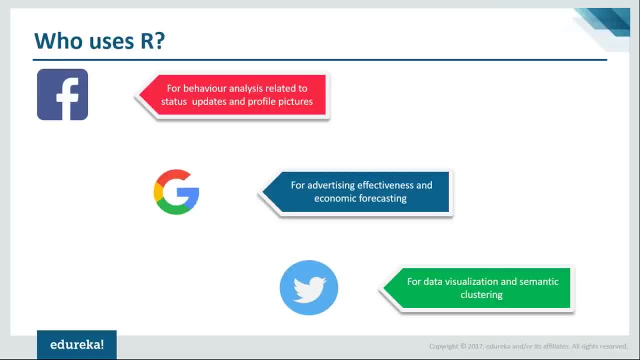 shots. the top-notch companies use R. Facebook users are for behavior analysis, Google users are for advertising effectiveness and Twitter users are for data visualization. So if your idea is to do some data science tasks, then R is definitely the programming language that you need to use. 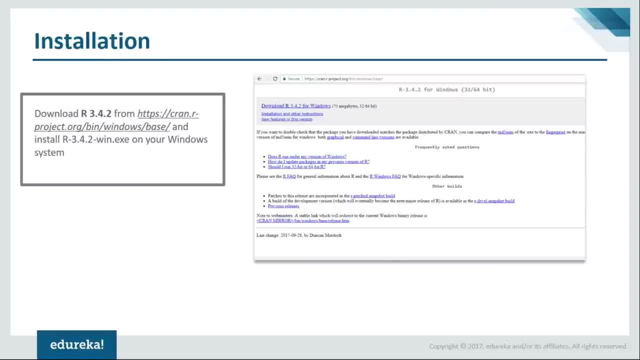 So you understood why R Who uses R? Let's finally go ahead and install R. So this is the site from where you'll be installing R. CRAN dot R hyphen project. Let's go to the CRAN repository, So I'll 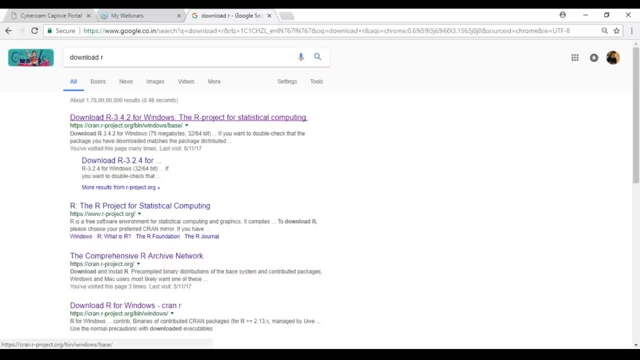 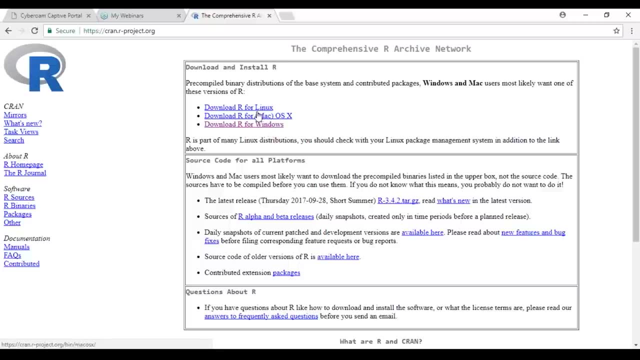 just type out download R over here. I'll click on the first link. If you have a Windows system, you can download R for Windows. If you have a Mac, you can download R for Mac. If you have a Linux, you can download R for Linux. Since I have a Windows system, I'm downloading it for Windows. 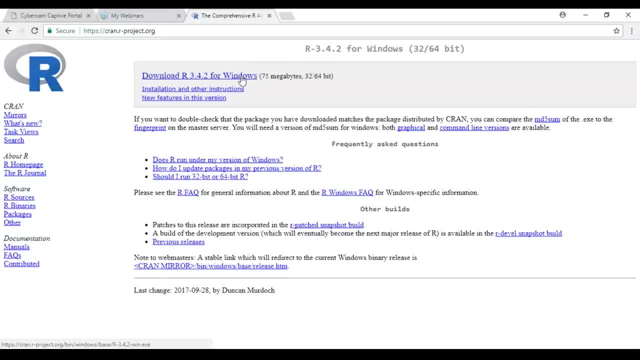 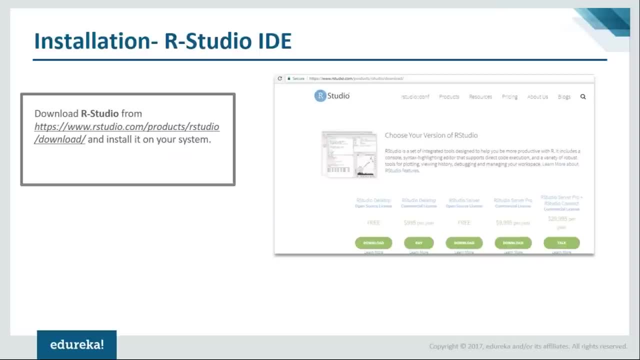 This is the latest version of R 3.4.2.. I click on download and the download starts. Now we also have an IDE, which is R Studio. Now I'd recommend all of you to also download the IDE before you perform programming, because R Studio makes our task easier. Let's go ahead and also download. 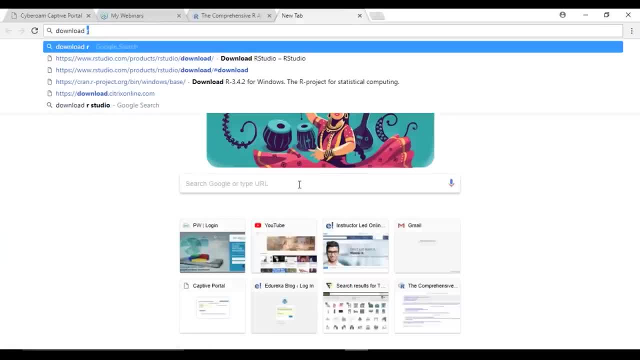 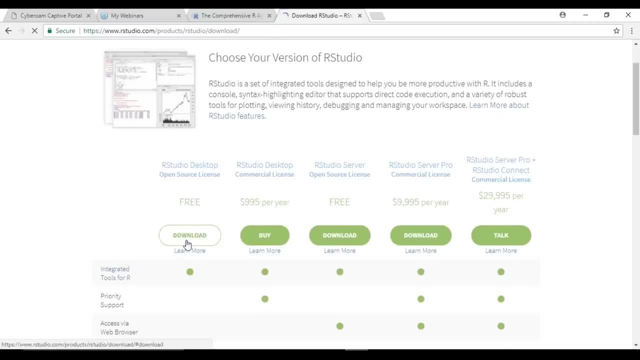 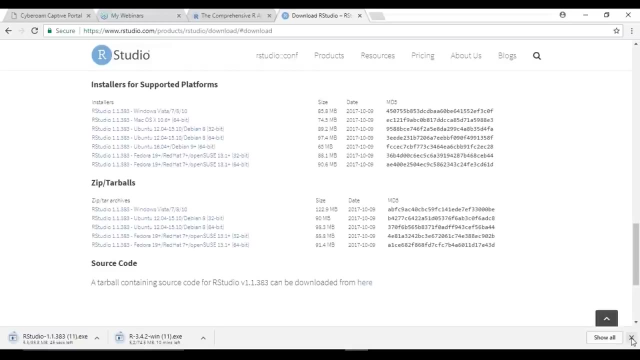 R Studio. I'll just type out download R studio here and click on the first link and it redirects me to rstudiocom. I'll download R studio, the free version, and these are the options: Windows, Mac and Ubuntu. I downloaded it for the Windows system and download starts. 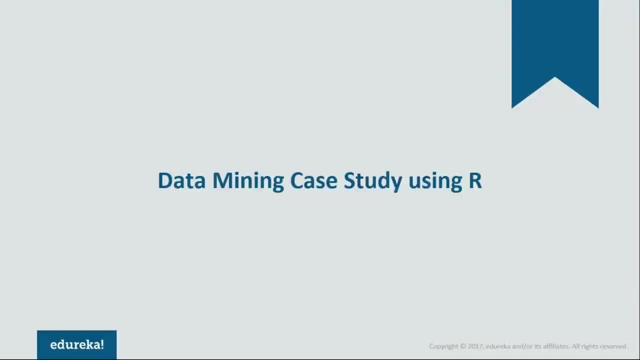 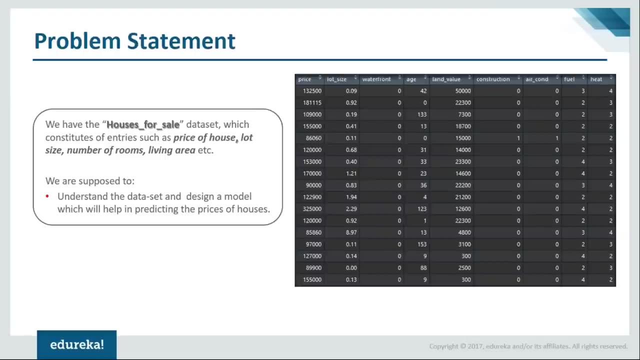 Now, since I've already installed R and R Studio, I don't need to install it again, So we'll directly go ahead to the key study. This will be our key study. We have the houses for sale data set, which comprises of price of house lot size. 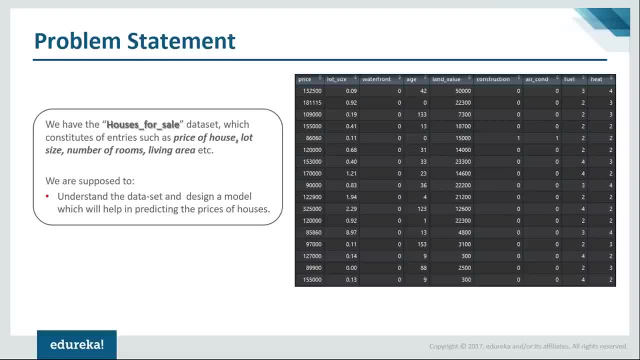 number of rooms, living area and so on, And our task is to understand the data set and design a model which will help us to predict the prices of houses with respect to other variables. Let's look at the tasks which we'll be performing in the key study. 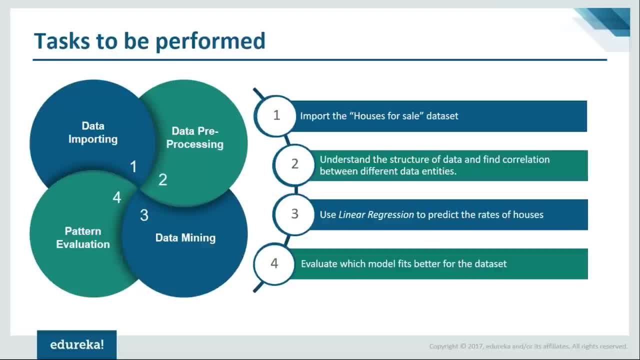 We'll start off by importing the data set and then we'll do a bit of pre-processing. The pre-processing will consist of understanding the structure of data and it will also involve a bit of data cleaning, because the data would be untidy. So we're supposed to make it tidy. 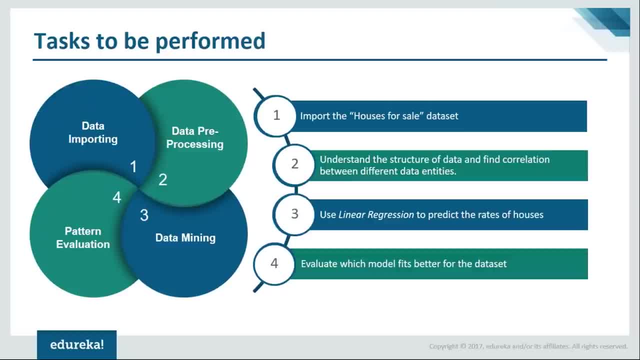 Then comes the important part, which is data mining, and the data mining technique which we'll be using is linear regression. So we'll use linear regression to predict the prices of houses and we'll be building two models actually, and out of those two models, we'll try to understand which model is more accurate. 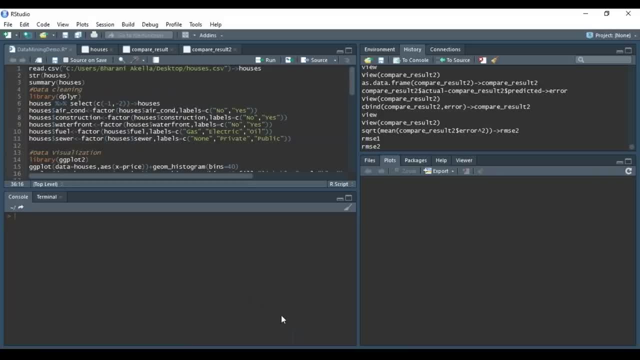 or which model will give us better results. Let's start with the hands-on session. This is our studio and this is how it looks like. This is a script window. this is the console window. Let's start with the first step. So, readcsv, this is the function with which we are importing. 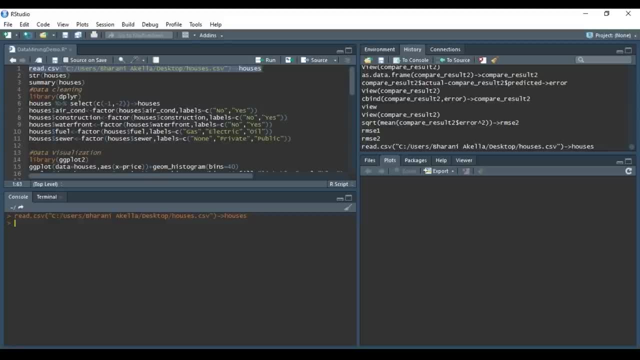 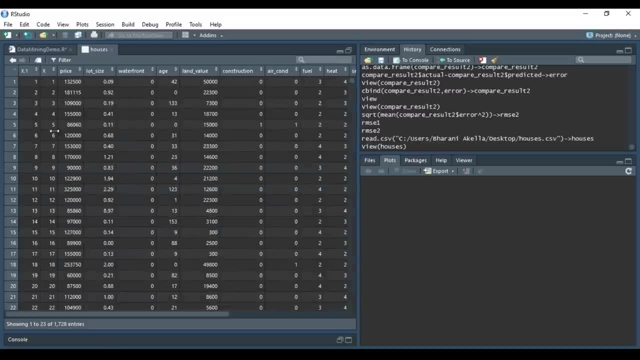 the csv file, and that csv file consists of the house's data set. Let's look at this data set. This is the data set, guys. So these two columns are so purpose? They just are numberings, So we would have to delete them. 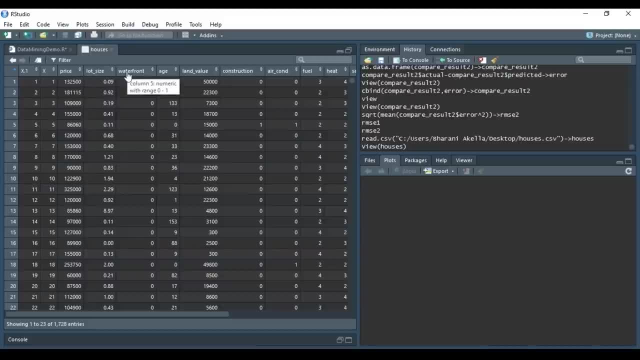 This is the price of the house. This is the lot size. This column tells us if the house has a waterfront or not. This column tells us how old is the house. This is the land value. This column tells us if the house. 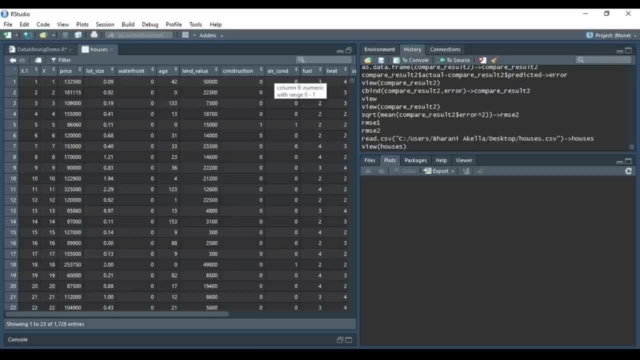 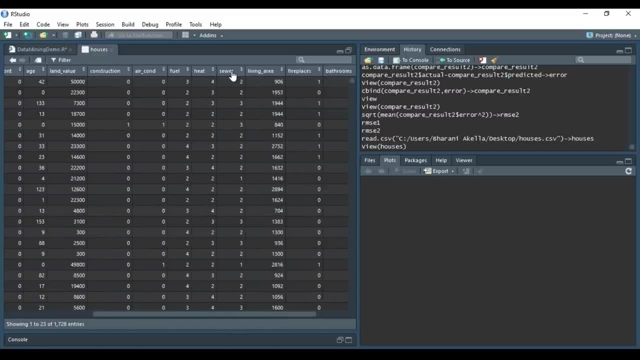 is newly constructed or not, And this is for if the house has centralized air conditioning or not. These two are the fuel types and the heat types used in house. This is the sewer system, living area, the number of fireplaces, number of bathrooms. 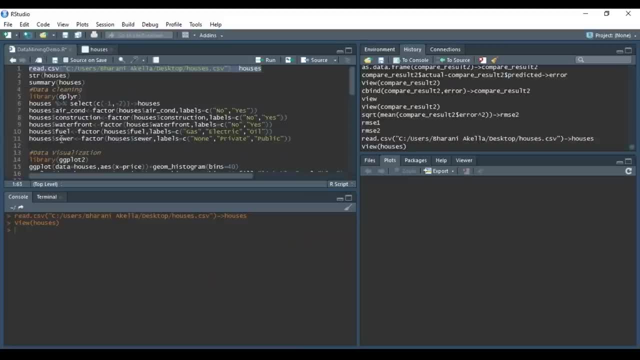 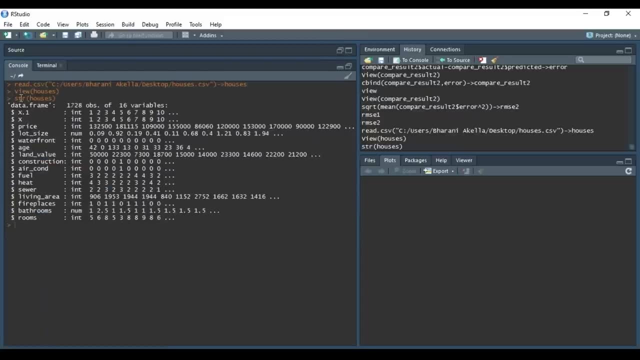 and number of rooms. That is the data set. Let's also look at the structure of the data set: STR function. with the help of STR function, we can understand the structure Now. this tells us there are 1728 observations and 16 variables in total. 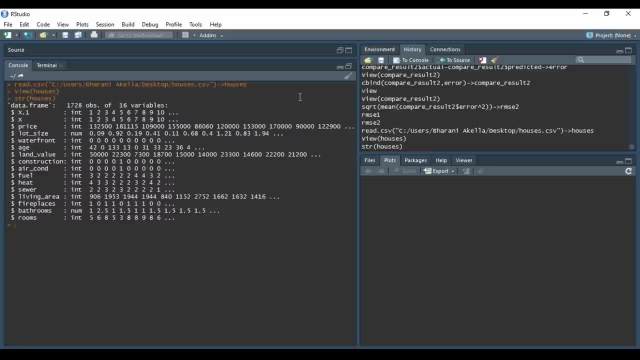 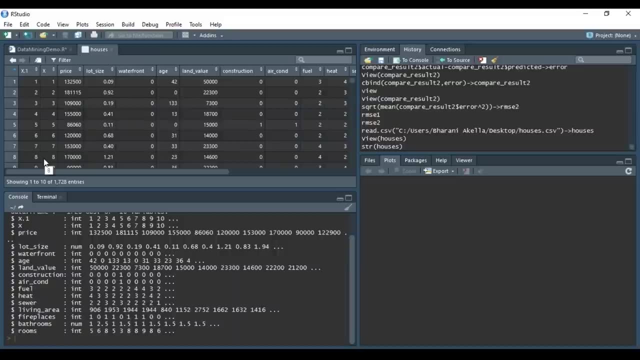 And most of these variables are of the type integer. That was the structure. Now we've understood that this data is not clean, So let's go ahead and do the pre-processing or a bit of cleaning. So the first task would be to delete these two columns. 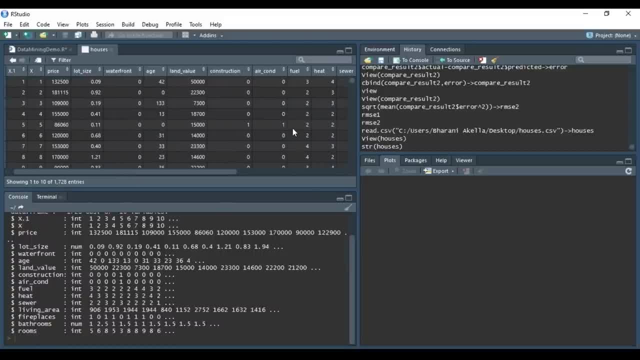 After that. now these values seem to be a bit ambiguous. So if the house has a waterfront, we can change it to yes instead of one, And if the house does not have a waterfront, we can change it to no instead of zero. 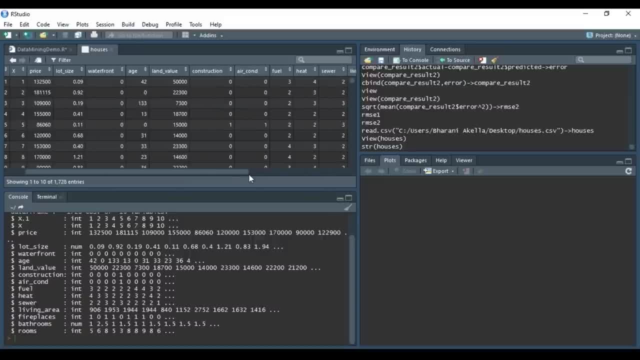 Similarly, we can change the values to yes and no for construction. Similarly, for the fuel type: instead of two, three and four, we can change it to electric gas and air. And again for the heat type, we can change it to hot air, hot water and electric. 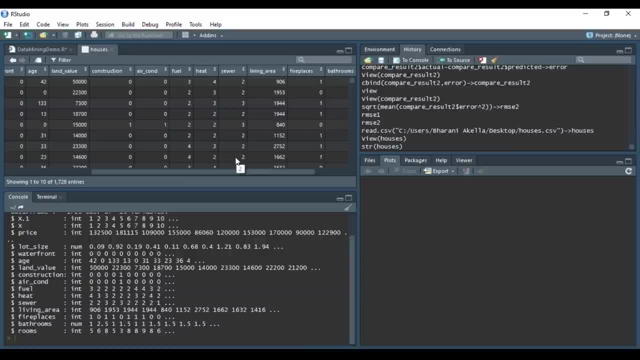 For the sewer system, it again has the values two, three and four. So instead of two, three and four, we can make the sewer system type to be private, public and none. So none will say that the house does not have. 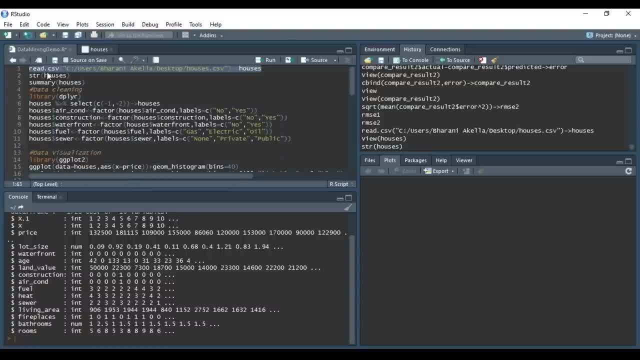 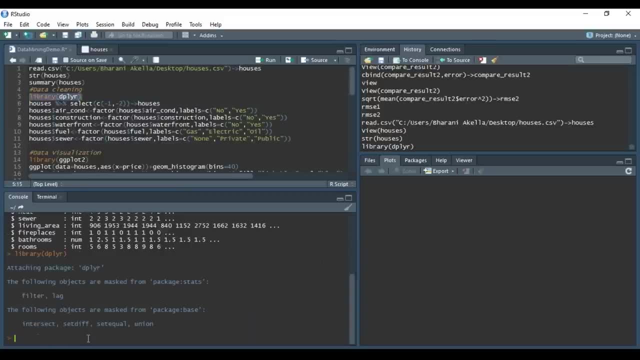 a sewer system associated with it. These are the basic pre-processing, pre-processing tasks that we would need to do, And for that we would have to load the deployer package. I'm loading it Prior to loading any package we are supposed to install it. 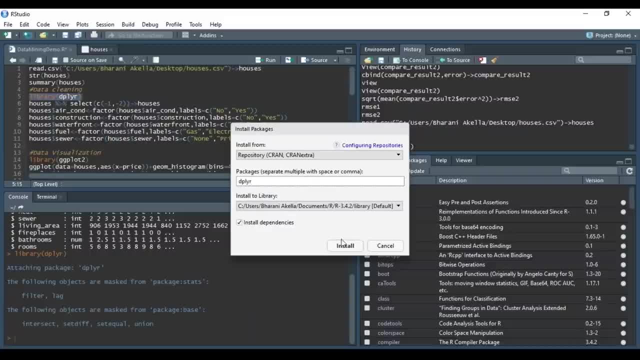 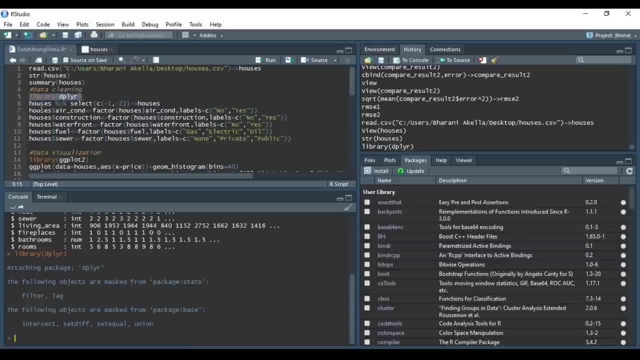 I click on install over here, I type out deployer, select it. Now, when I say install, the package will be installed. And since I've already installed the package, I don't need to do it again. I've loaded the package. 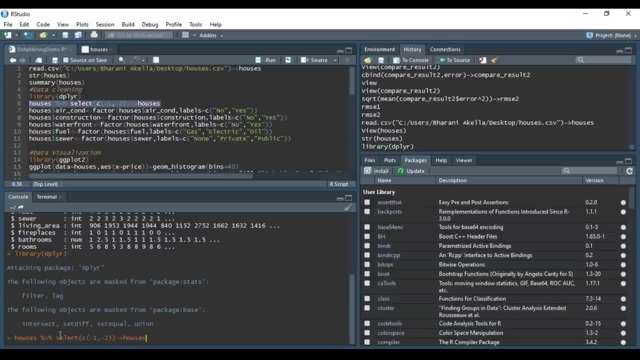 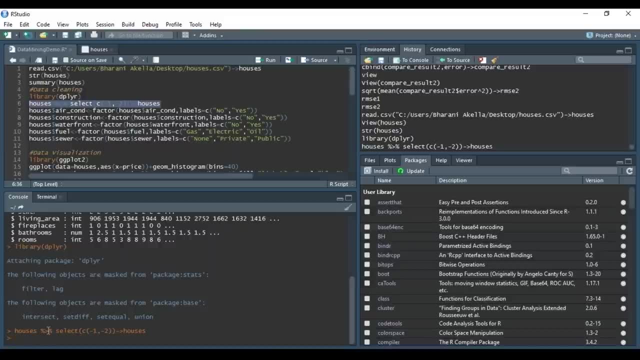 Now it's time to delete the first two columns. The select function comes from the deployer package and this is the dataset. And this symbol over here that you see is the pipe operator. The pipe operator helps us to connect things. So from the house's dataset. 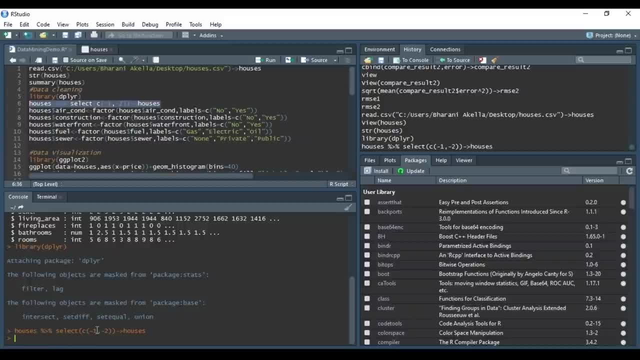 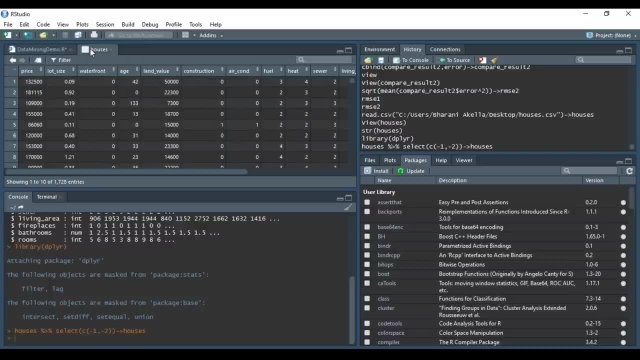 we are selecting all other variables except the first and the second column and we are storing the result again in the house's dataset. So we've applied the command and we see that the changes have taken place. The first two columns have been deleted. 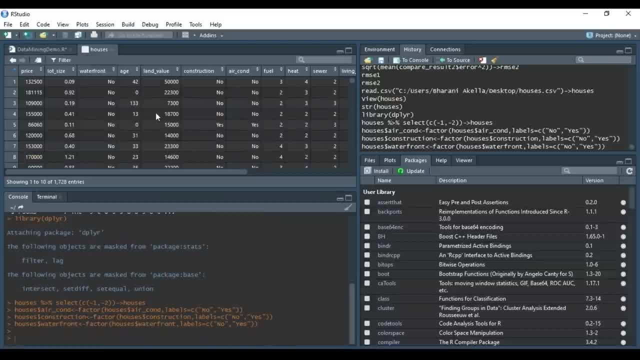 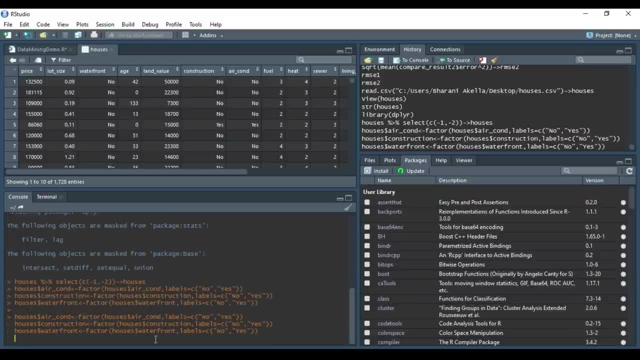 Let's go ahead with the pre-processing. We saw that wherever the values were zero- one, two, three and four and five and six, Zero and one- they have been changed to no and yes, Let's again have a look at these commands. 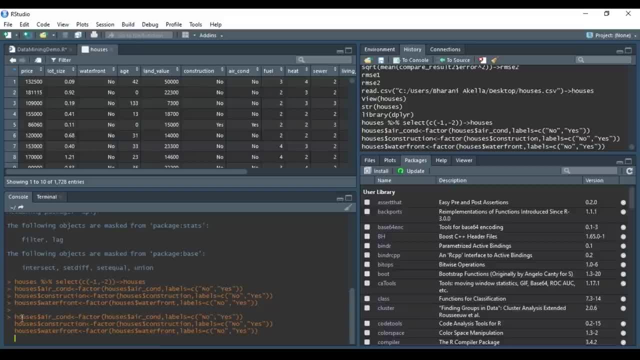 So dollar symbol helps us to select the column. So, with the help of houses dollar aircon, what am I doing is I'm selecting the air condition column of the house's dataset. So I select this column and I change it to a factor. 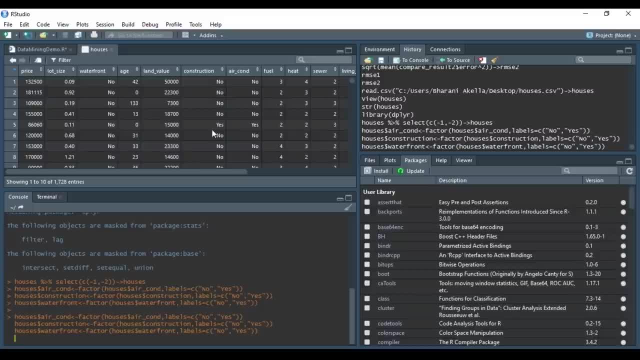 that is initially the values for numerical. Now I'm changing it to a categorical variable. I've changed it to a categorical variable and now it's time to change the labels of it. So initially the labels were zero and one, and I'm changing the labels to no and yes. 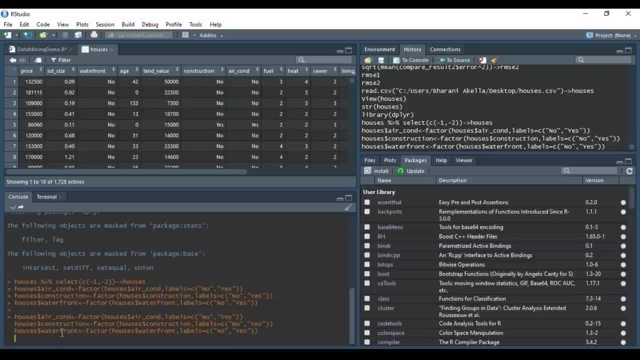 I've done the same for construction column and waterfront column. So I've selected the construction column, changed it to a categorical variable and changed the labels to no. and, yes, I've done the same for the waterfront column as well. Now let's go ahead and also change the fuel type. 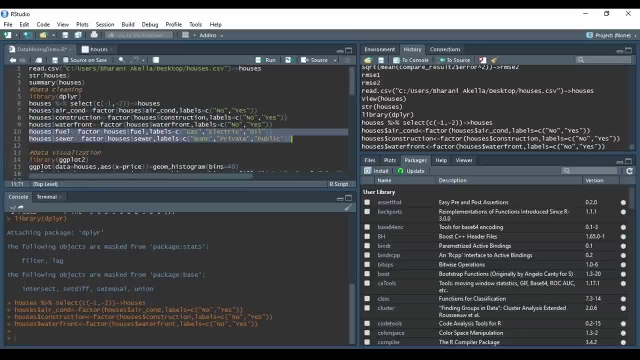 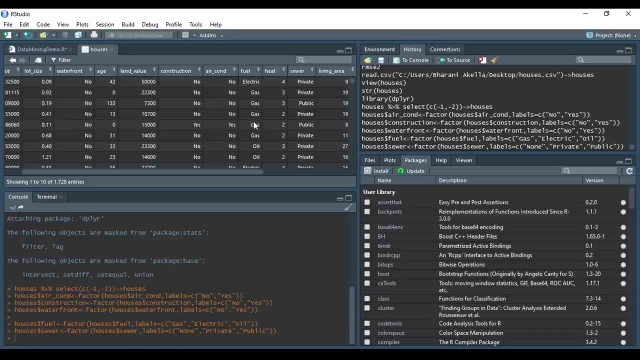 heat type and the CO system. Let's go ahead and do that. I've changed the fuel and sewer, So the fuel type has been changed to gas, electric and oil, and the type of sewer system has been changed to non-private and public. 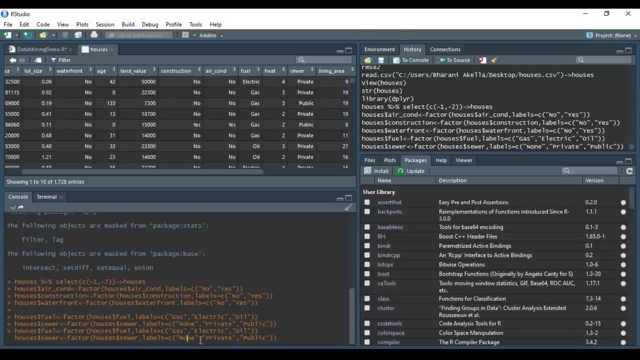 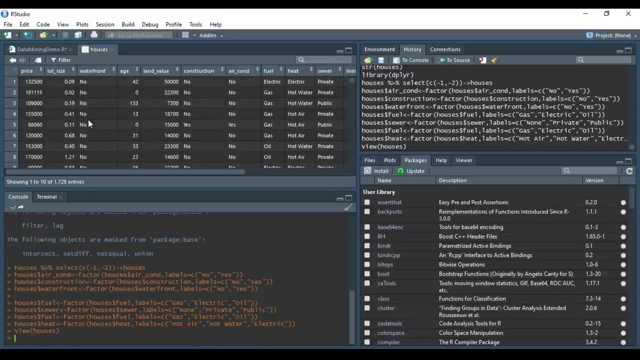 We also need to change the heat column. Let's also do that. So I'm selecting the heat column with the help of the dollar symbol. I'll change to hot air, hot water and electric and the changes will be applied. Yes, the changes have been successfully applied. 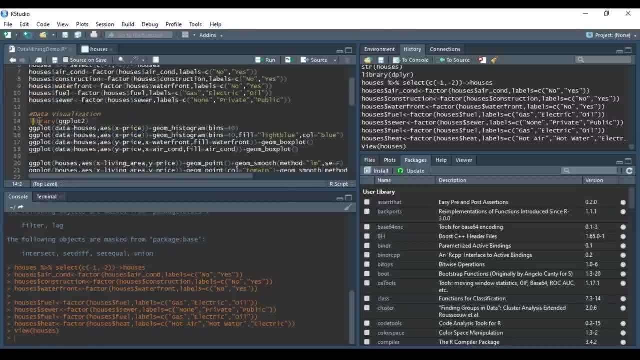 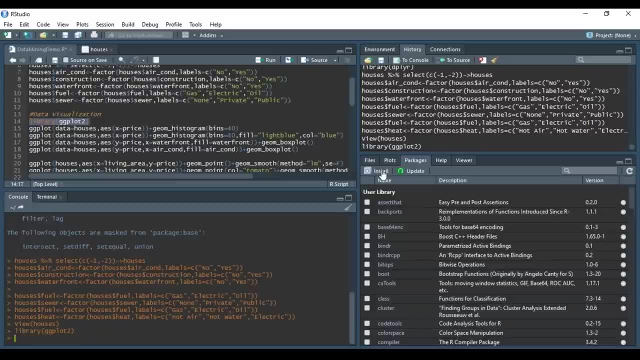 We're done with the pre-processing. Now let's start visualization. For visualization R provides us with a package which goes by the name of ggplot2.. And again, prior to loading the package, we're supposed to install it. I just type out ggplot2 over here, select it. 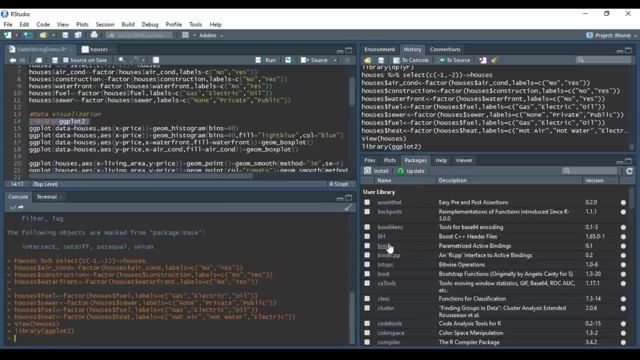 and when I click on install, the package will be installed, And since I've already installed it, I don't need to install it again Now. ggplot2 is based on grammar of graphics. Now, whenever we are trying to form a sentence, 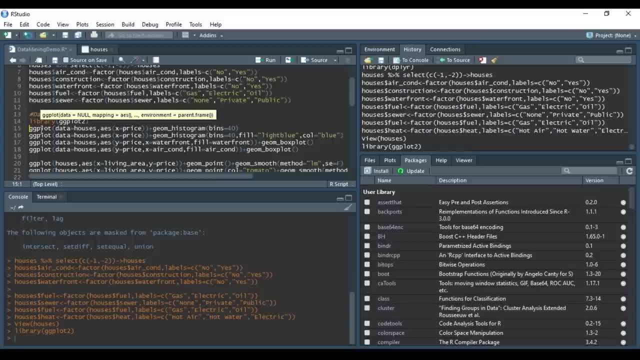 we are supposed to follow the grammatical rules. Similarly, whenever we are making graphs, we have something known as grammar of graphics and we need to follow this grammar of graphics. Let's understand what exactly is grammar of graphics. So, for this command, grammar of graphics has three parts. 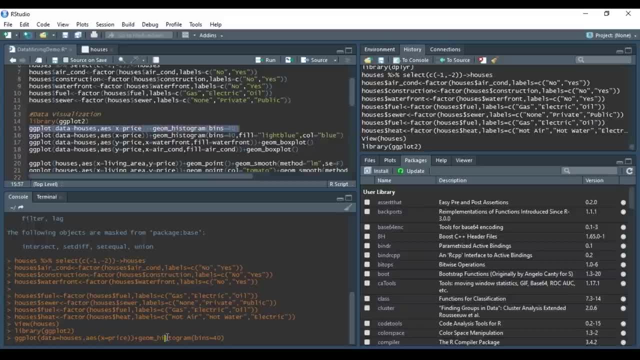 The first is the data part, Next is the aesthetic, Next is the geometry. So first we're supposed to select the data set on which we're supposed to do the plotting. So over here I've selected the houses data set. Next are the aesthetics. 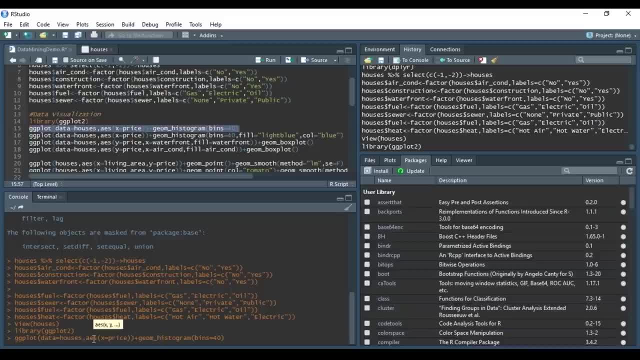 So aesthetics tell us on what variable are we supposed to map. That is, we can select the aesthetics, such as x-axis, y-axis, or the color or the fill or the size of it. So these are the aesthetics and we assign variables to these aesthetics. 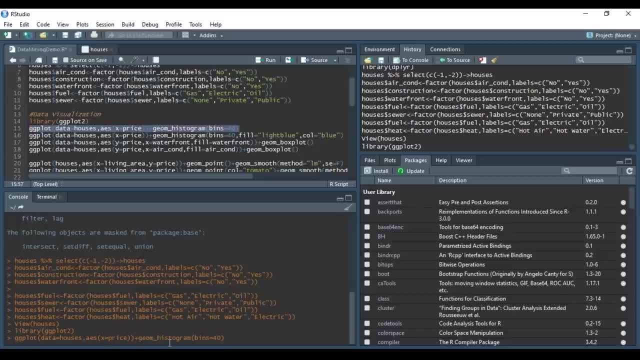 So for this case, I've assigned the price to the x-axis. And then, finally, it's time to decide the geometry, that is, the type of graph that we want to plot. We can either select a histogram box plot, scatter plot or a line plot. 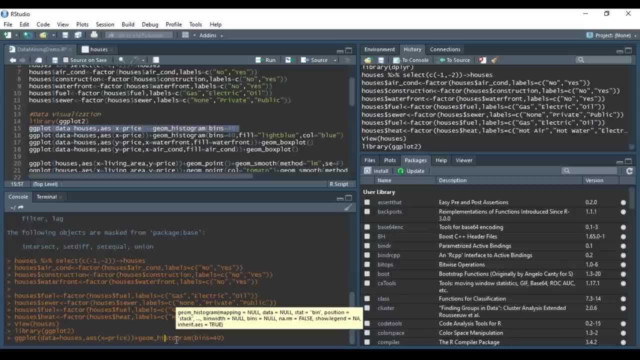 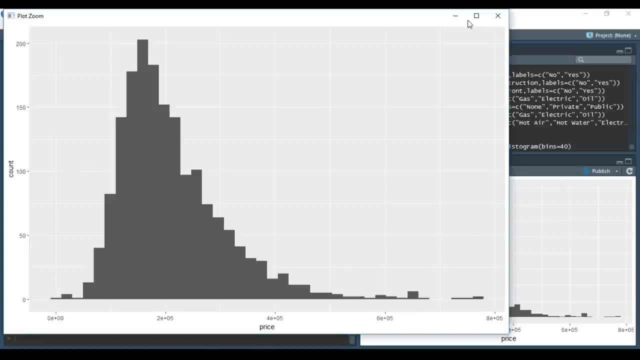 So, whatever is our need, we can select a geometry for that. So now I would want to know what is the distribution of price. Let's plot this. I've plotted the graph. Now this is the price distribution. You see these values over here. 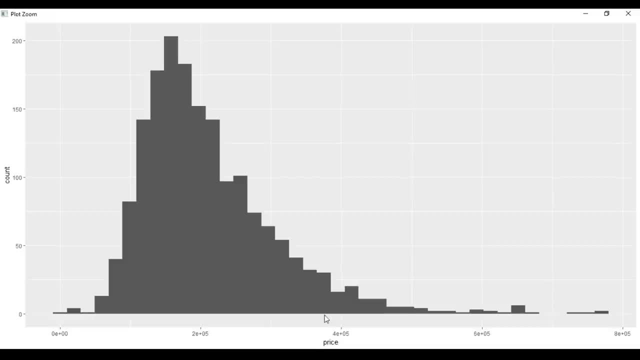 So this is 2e plus 0.5, 4e plus 0.5, 6e plus 0.5.. That basically stands for 2 into 10,000.. 4 into 10 power 5,. 6 into 10 power 5.. 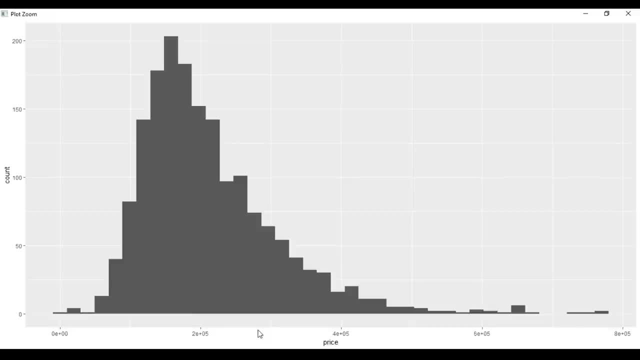 That again means the value is around two lakhs, four lakhs or six lakhs and eight lakhs. So from this graph we can infer that the average salary of the houses is around two lakhs and the maximum price of the house 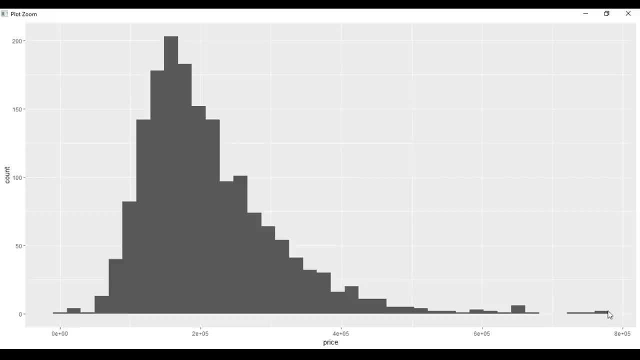 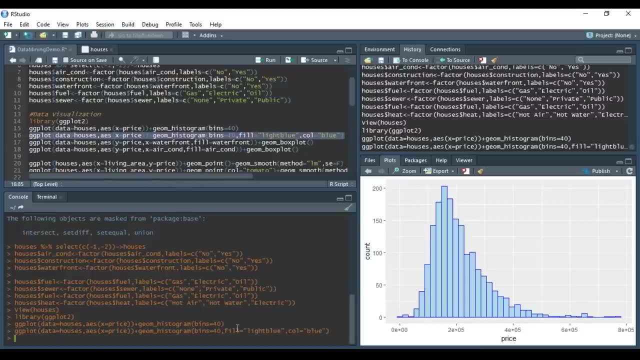 would be around somewhere close to 7.5 lakhs. We're done with this. Let's add a bit of color to the plot so that it looks prettier In the geometry. I've added two more attributes: I have fill and I have color. 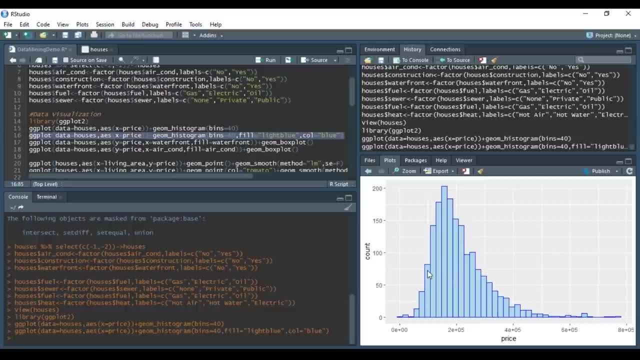 So the fill is of light blue and color, which is the boundary, is of dark blue. So the same graph. I just added color to it. Now let's understand. how does price vary with respect to waterfront, That is, if the house has a waterfront? 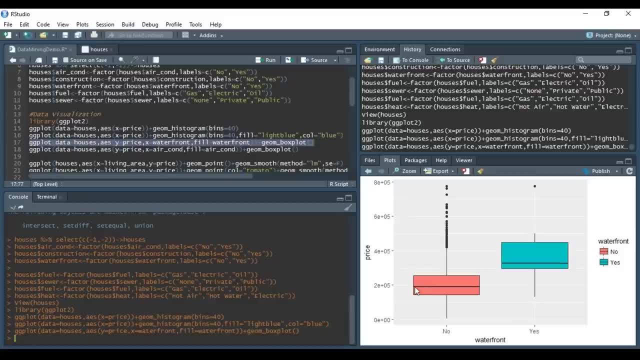 what is the price of the house? And if the house does not have a waterfront, what is the price of the house? So the data is again: houses. The y-axis denotes price, X-axis denotes whether the house has a waterfront or not. 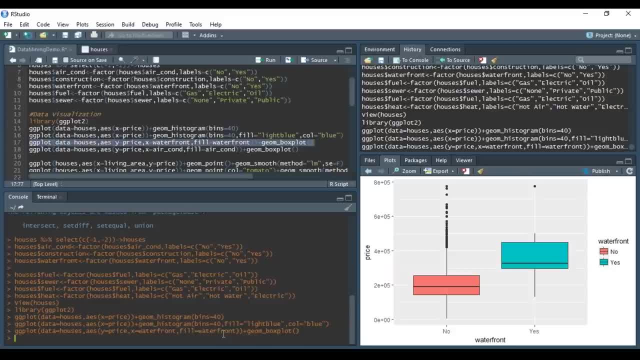 and the color is again determined by whether the house has a waterfront or not, And the geometry used over here is boxplot. So the color or the fill is automatically determined by the variable. Since waterfront has two categories, it gives two colors. 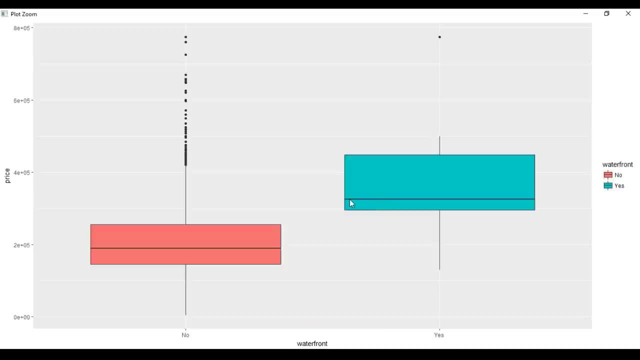 Let's look at this So we can easily infer that if the house has a waterfront, it will have a higher price, and if the house does not have a waterfront it will have a lower price. So we'll be comparing the median values. 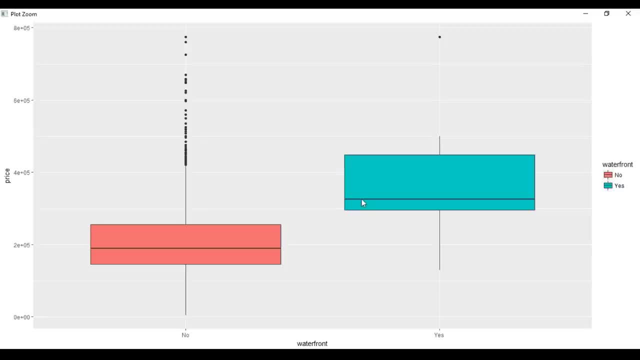 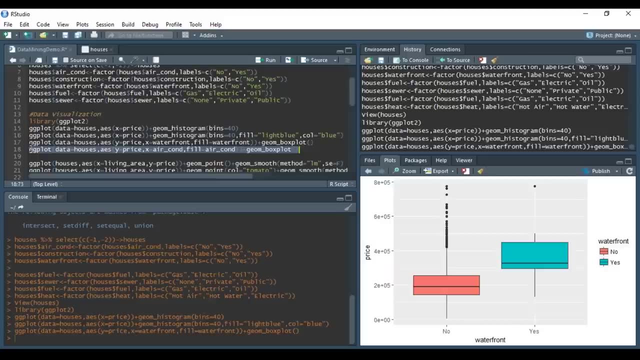 just to be sure. So this: the median value of the house which has a waterfront is higher and the median value of a house which does not have a waterfront is lower. Now let's see. how does the price vary with respect to the air conditioning? 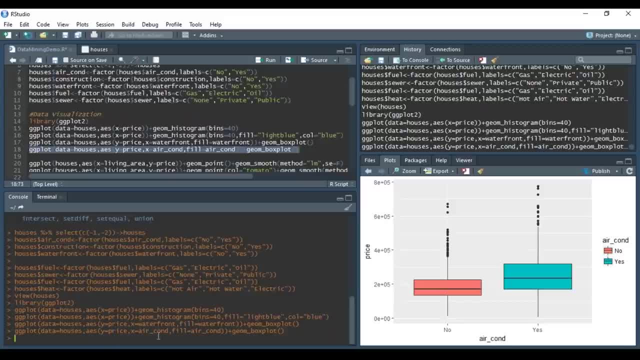 Again, data set is houses. Y-axis is price. X-axis is determined by whether the house has air conditioning or not. The fill is determined by, again, whether the house has air conditioning or not. Geometry used is boxplot. Again, we can very easily infer that. 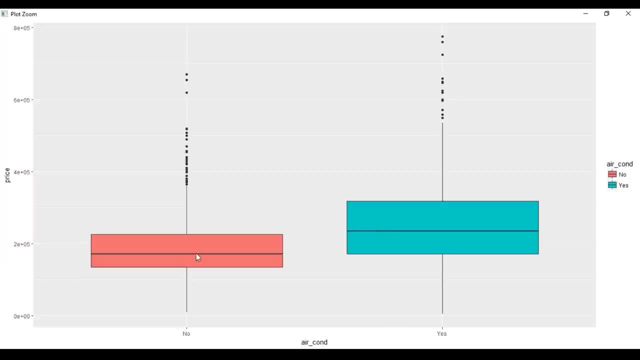 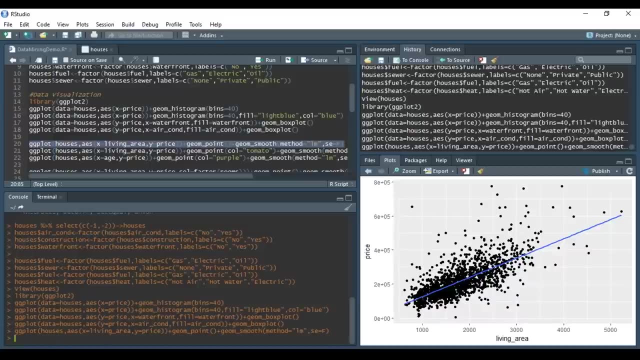 if the house has air conditioning, its price will be higher, and if the house does not have air conditioning, its price will be lower. Let's see: how does price vary with respect to living area? So over here, the geometries used are scatterplot. 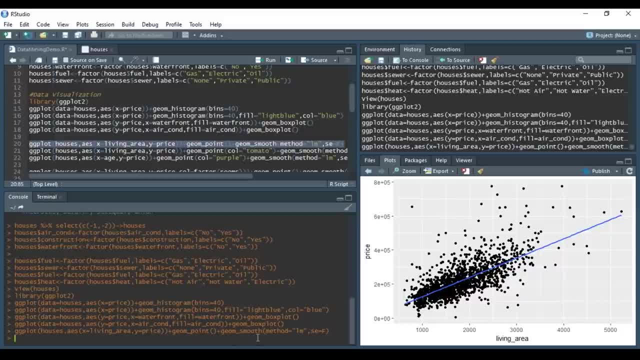 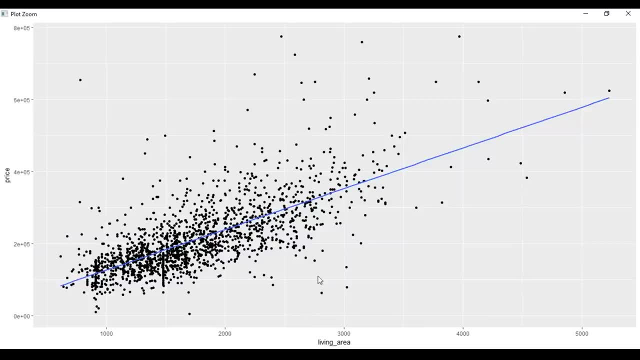 and a lineplot. So germpoint is for scatterplot, Germsmooth is for lineplot, And again X-axis is for living area, Y-axis determines the price. So we see over here that it is a linear relationship. 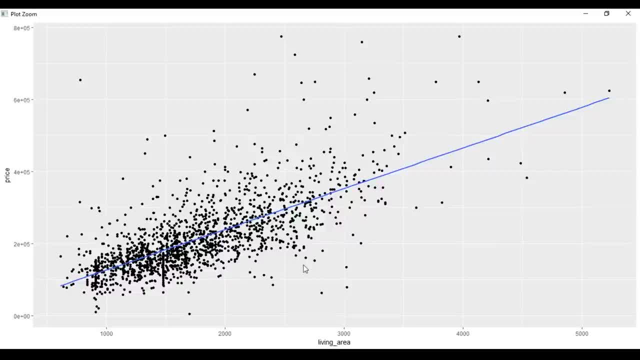 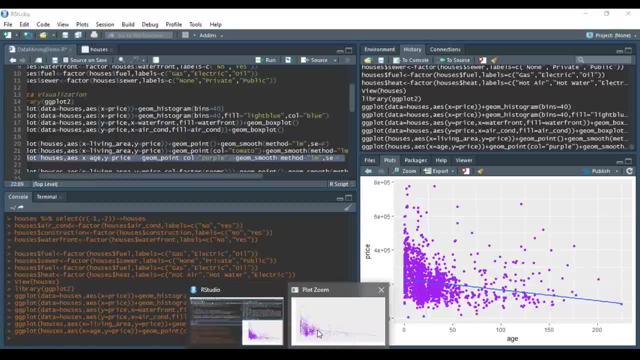 That is, as the size of living area increases, the price of the house also increases. Now let's see: how does the price vary with respect to the age of the house? Now, this is inverse relationship, That is, if the age of the house increases, 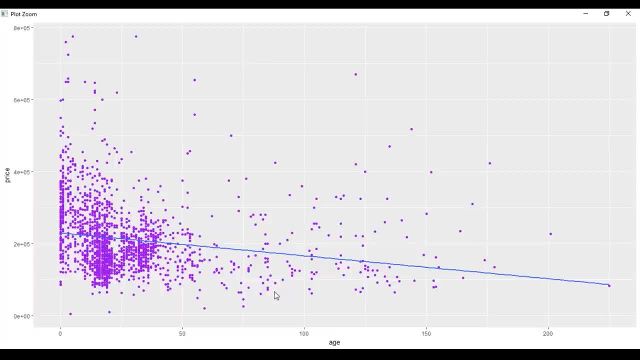 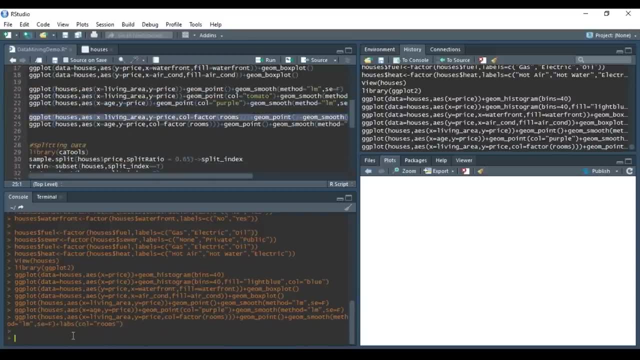 that is, if the house is old, its price will be low, And if the house is new, its price will be high. This will be a very interesting plot. Quite a pretty plot, isn't it? Again, Y-axis determines price. 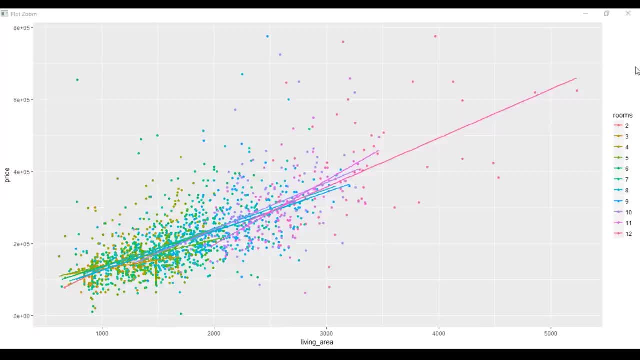 X-axis determines the size, The price of living area And this over here that you see, is that the colors are determined by the number of rooms. So if the house has five or six rooms, then the price of the house would be around 1.5 lakhs. 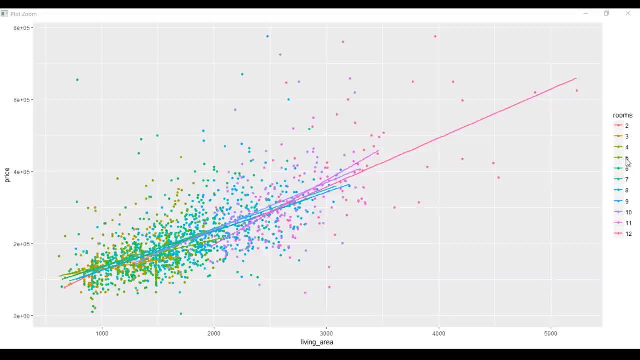 to 4.5 lakhs, because the color of the house, if it has five or six rooms, is green, And all of these green dots come between 1.5 lakhs to 4.5 lakhs. Similarly, what we can say is if the house has 12 rooms, 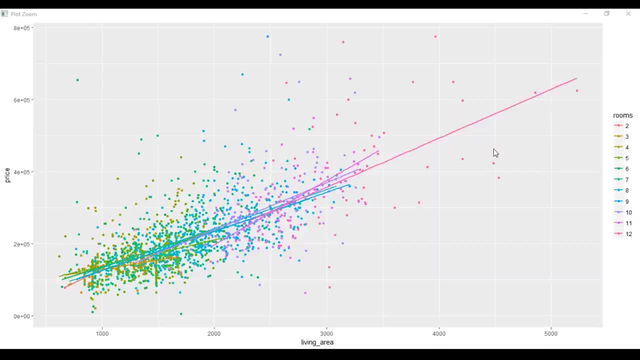 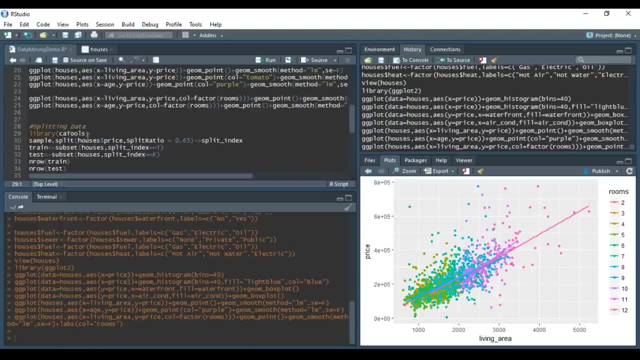 so it will have the maximum price. So these are the sort of inferences which we can make from this graph. To select the data, we've done a bit of cleaning. We've also done a bit of visualization. Now it's time to come to the most important part. 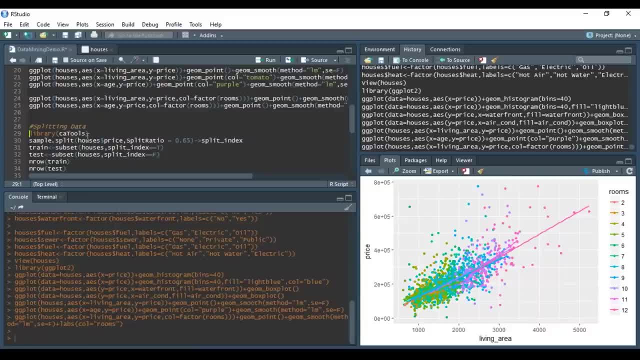 of the case study which is applying the data mining technique. Now, prior to building the linear regression model, we're supposed to split our data into training set and testing set. We do this because this helps us to measure the accuracy of the model built. 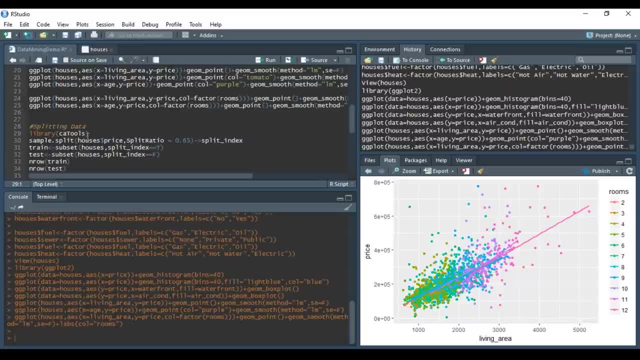 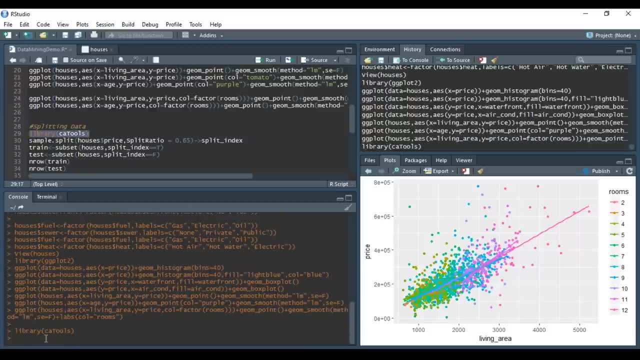 So we build our model on the training set and check for its accuracy. on the test set To split the data set, we're supposed to load the CA tools library, the CA tools package, And again so, prior to loading, we're supposed to install the package. 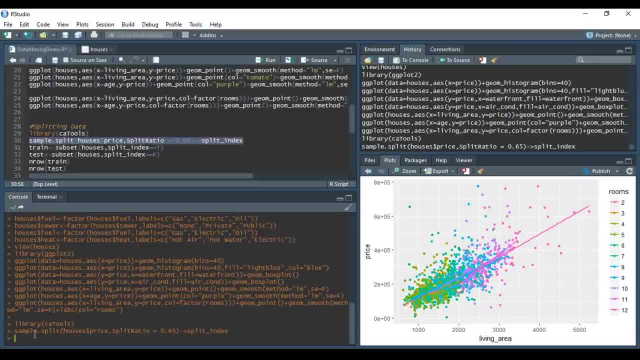 CA tools package provides us with a function which goes by the name of samplesplit. Now this has a parameter: split ratio. Split ratio determines how many of the observations get true and how many of the observations get the false label. So we've given the split ratio to be 0.65.. 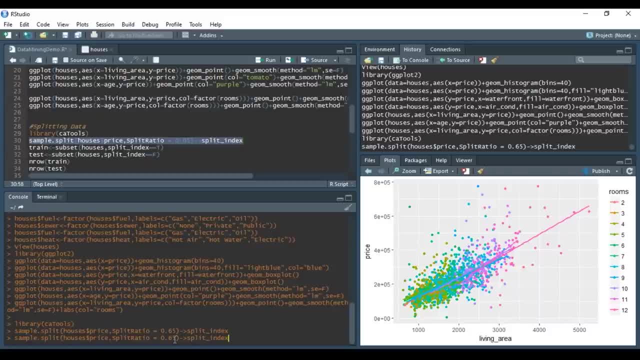 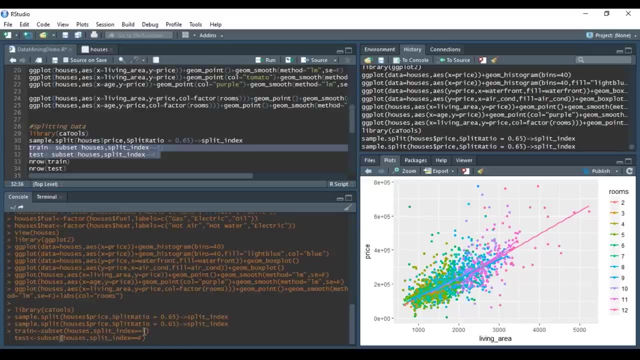 That is, 65% of the observations will have the true label and 35% of the observations will have the false label. And I've stood the result in split index Splitting is done. So what are we doing over here Now? wherever the value or the label of the observation, 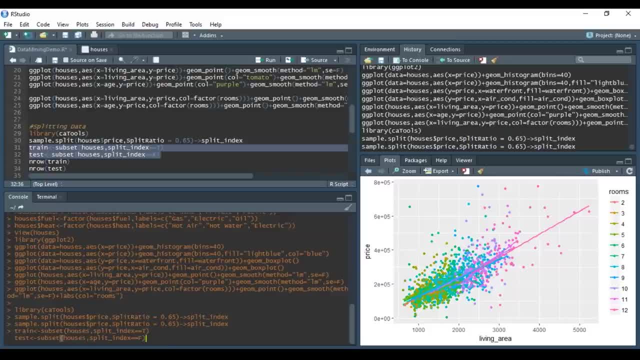 is true. we are selecting all of those observations and storing them in the training set. the value of all the observations is false. you're selecting them and storing them in the test set. So training set comprises of 65% of the observations and 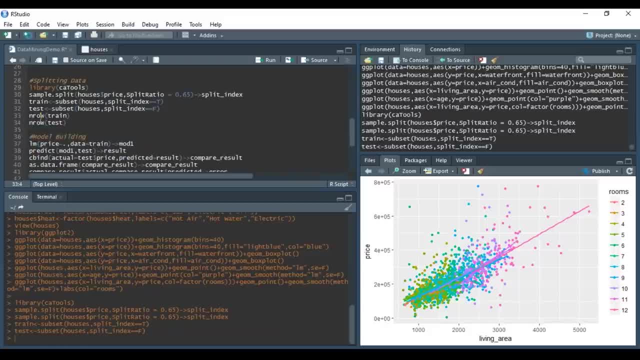 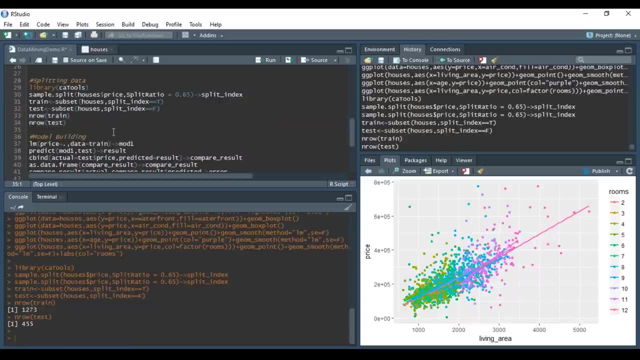 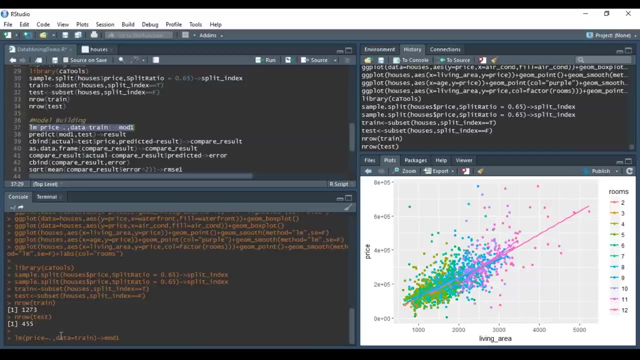 testing set comprises of 35% of the observations. Train set has 1273 rows. test set has 455 rows. That is the 65-35 split. You split the data. Now it's time to build the model. You're building linear. 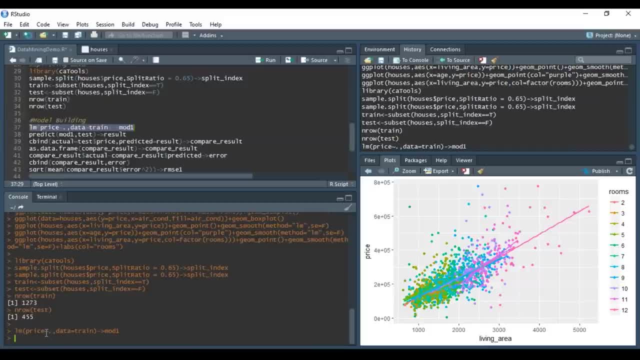 regression. So, as we saw, the basis of linear regression is a linear equation which is: y is equal to mx plus c. So over here. this is the formula. So the tilde symbol: on the left side of this tilde symbol we have the dependent. 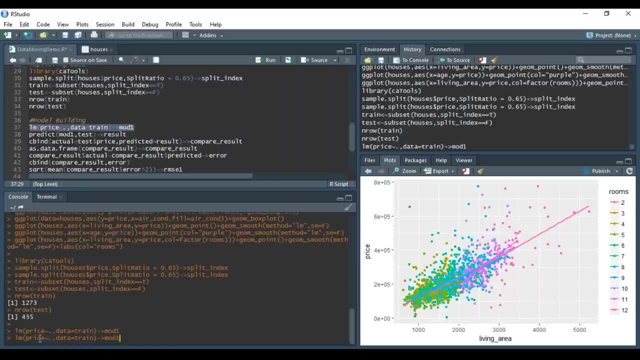 variable, and on the right side of the tilde symbol we have all the independent variables. So the price is the dependent variable, and when we put a dot over here, this basically determines that we are selecting all other columns except the price, That is. 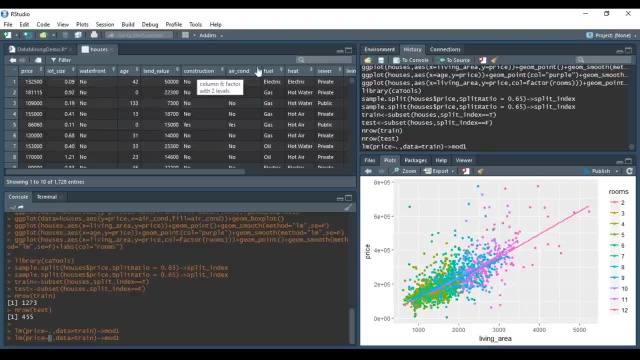 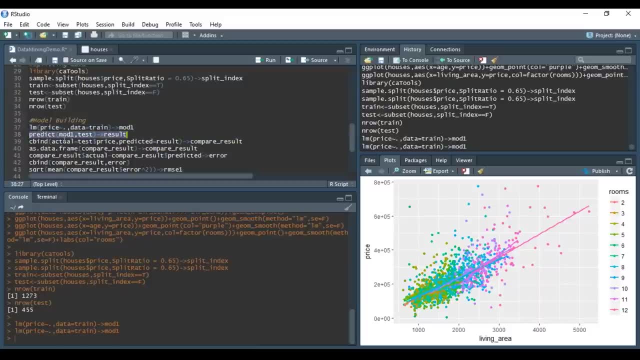 the target value. So we're trying to understand how does price vary with respect to all other columns in the data set? And we've built the model and stored it in the object mod one. Now it's time to predict on the test data set. So we check for the 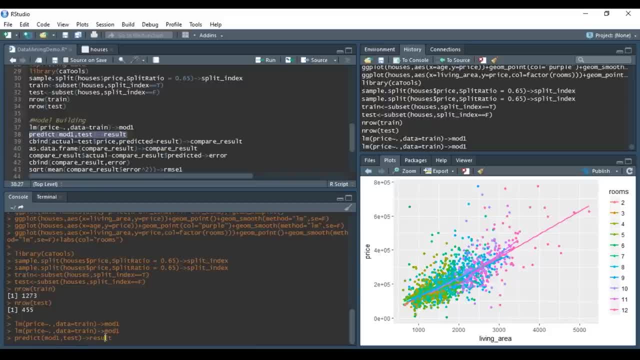 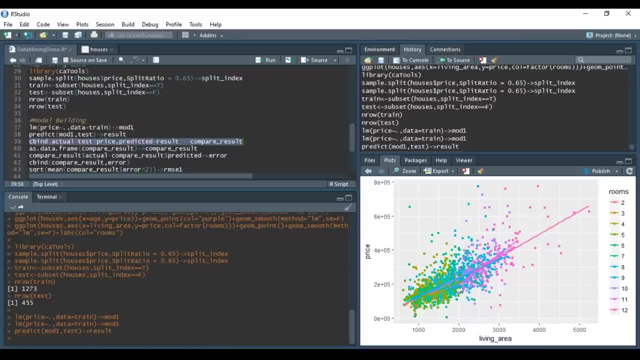 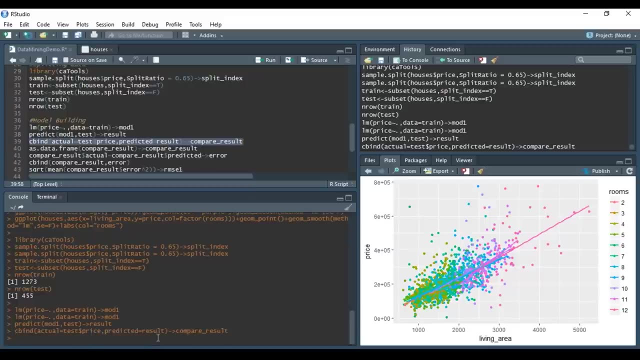 accuracy of it on the test set and store the result into an object which has the name of result. I do this. Now. let me bind the actual values and the predicted values, So the test set has the price column which I have. the actual values and the predicted values are in the result object, So I'm 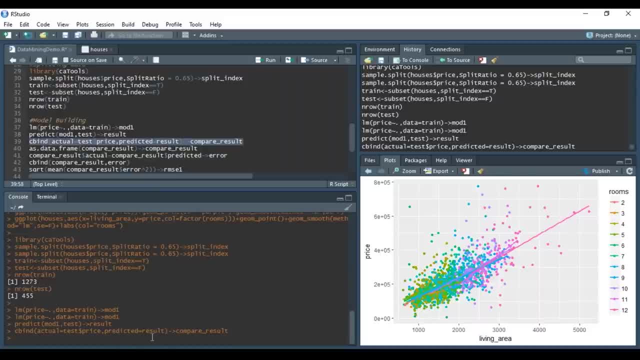 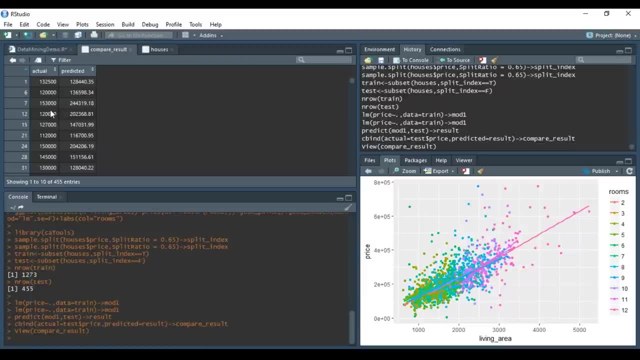 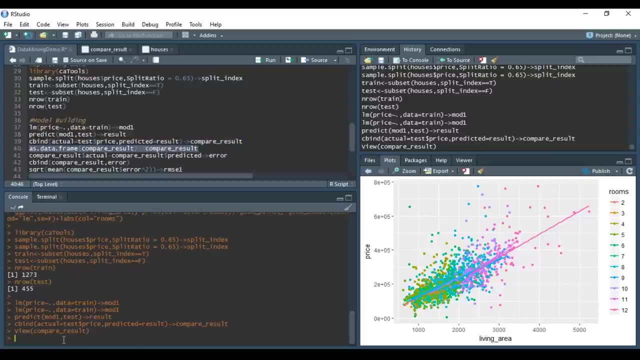 naming it as predicted, and I'm combining these two columns and storing it in an object whose name is compare result. Let me have a look at this. These are the actual values and these are predicted values. Let's find out the error in prediction Now. since compare result is a matrix, we're supposed to convert it to a. 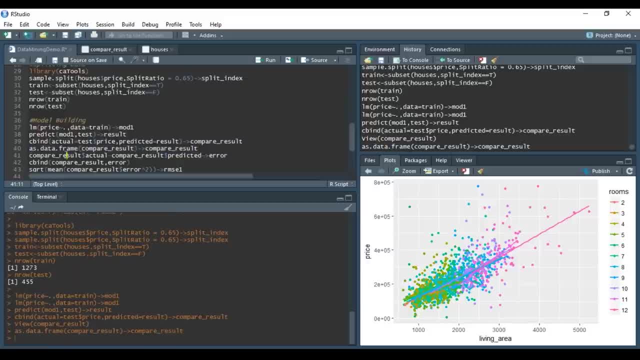 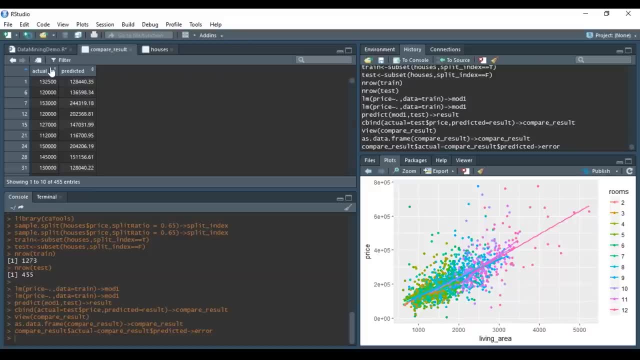 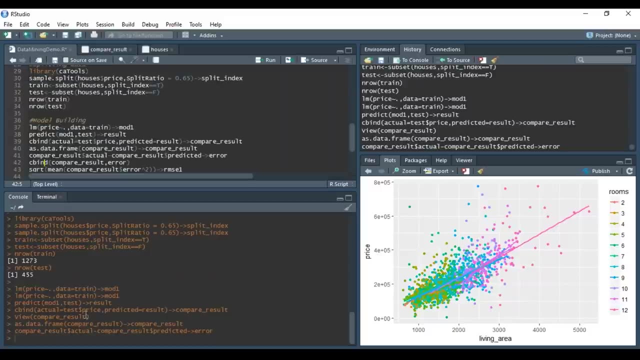 data frame using as dot data frame function. I've changed it to a data frame. I found out the error. So we find out the error by just subtracting actual values minus predicted values. So actual values minus predicted values gives us the error in prediction. That is what I've done over here. Let me also bind the. 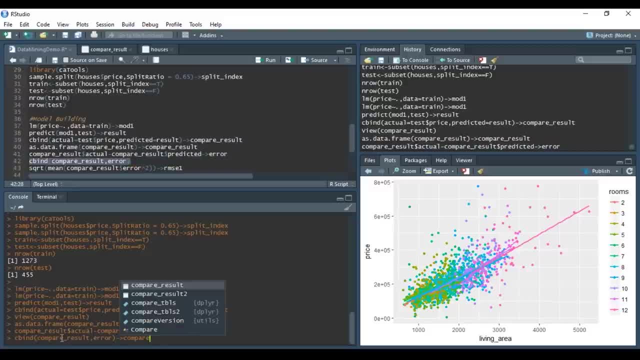 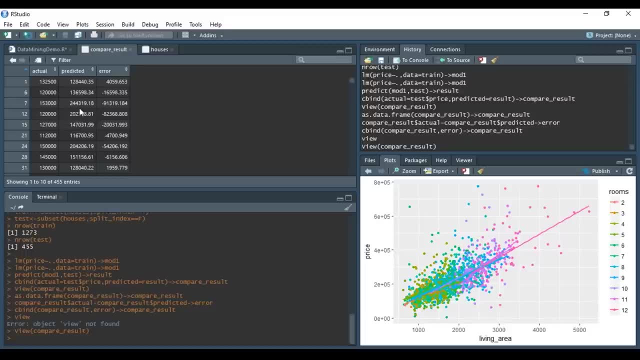 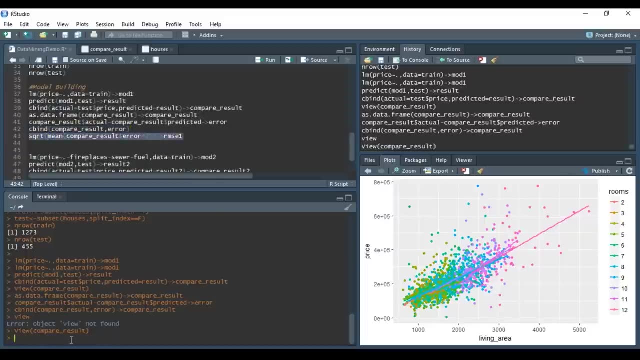 error in prediction to the same data set and store it in compare result. Let me have a look at compare result. So actual values, predicted values and error in prediction. We have something known as root means, square error. to check for its accuracy, We store it in rmsc1.. Let's look at its. 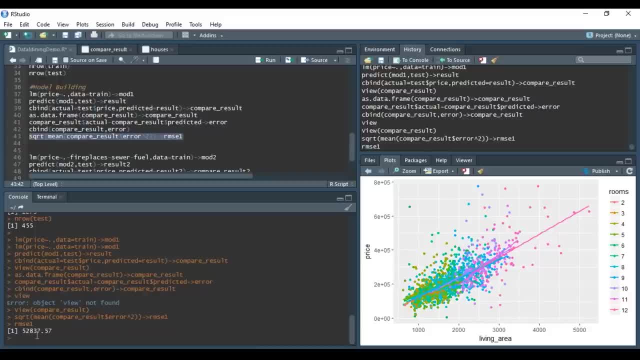 value. So this is the error in the prediction. 52 837.57 is the error in prediction. Now let's also have a look at the summary of the model built. So this was the model which we build on the training set and this is the summary. So 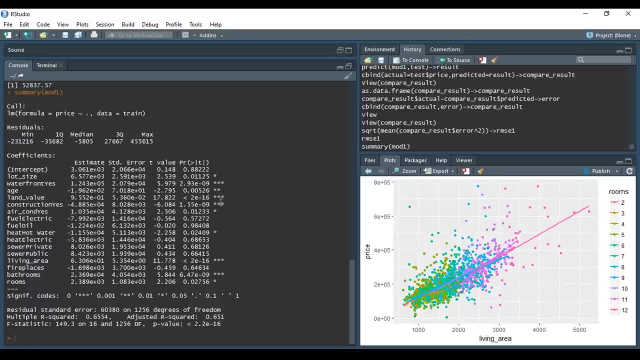 these stars which you see over here. These tell us how much is the impact of this independent variable on the dependent variable. Greater the number of stars, greater is the impact. So wherever the variable has three stars, that would mean it has a greater impact on the dependent. 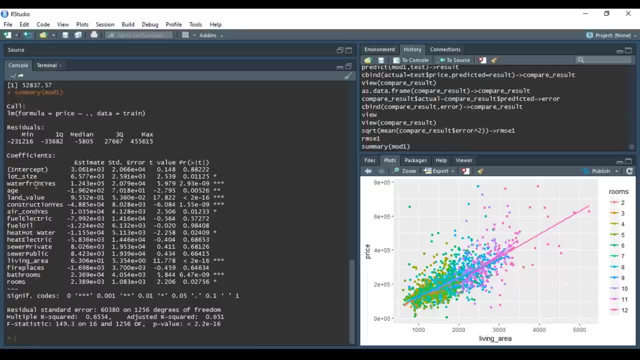 variable. So if the house has a waterfront, then it will have a greater impact on the price of the house, If the land value again has a greater impact on the price of the house, and if it's newly constructed, it again has a greater impact on the price. Now let's look at the opposite side, that which do not have. 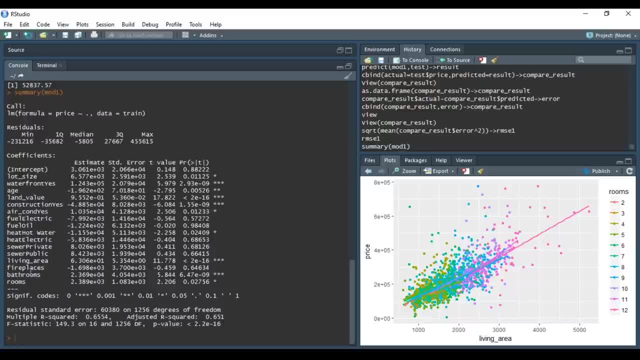 an impact at all. So heat, sewer, the number of fireplaces, the type of heat used or the type of fuel used or the number of fireplaces used, They do not have an impact on the dependent variable at all. We have another check for the accuracy of the model, which is: 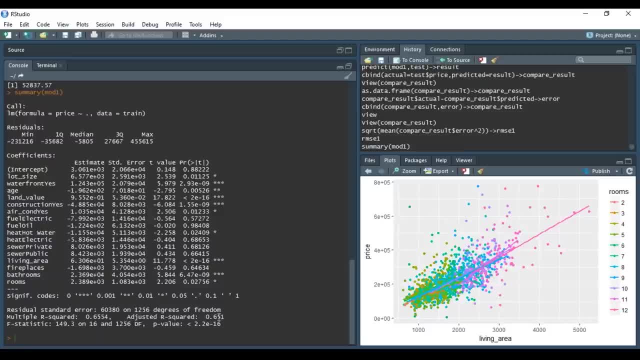 the adjusted R squared. So if this value is closer to one, then that would mean this model is perfect. So the accuracy of this model is around 0.651.. Now let's build another model and compare that model with this. This is the second model. 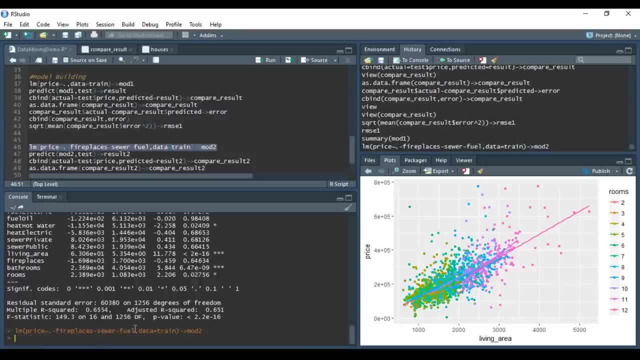 Now, since we've understood that fireplaces, sewer and fuel do not impact the dependent variable at all, So I've selected all other variables except these three variables. You see this minus symbol. So I'm removing fireplaces, sewer and fuel by putting a prefix minus before it. I'm storing the result in mod 2.. I predict the. 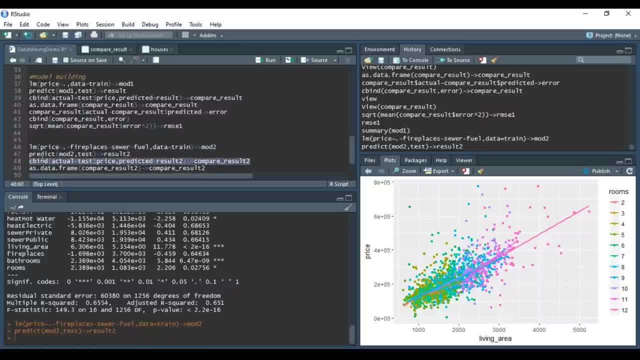 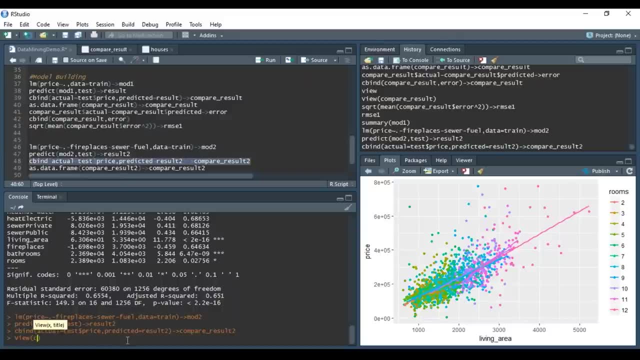 model on the testing set and store it in result 2.. Now it's time to bind the actual values and the predicted values, and I store it in compare result 2.. Let's have a look at compare result 2.. This is compare result 2.. These are the 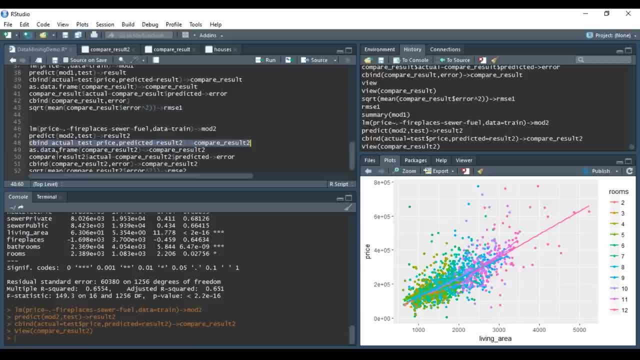 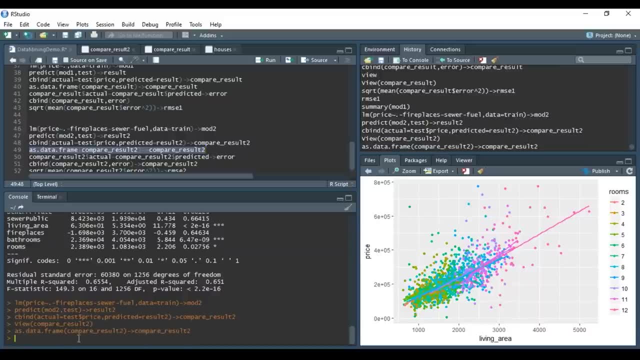 actual values and these are the predicted values. Let's have a look at the. yeah, we're supposed to change it to a data frame, since it's a matrix, So change it to a data frame using asdataframe. Now it's time to find out. 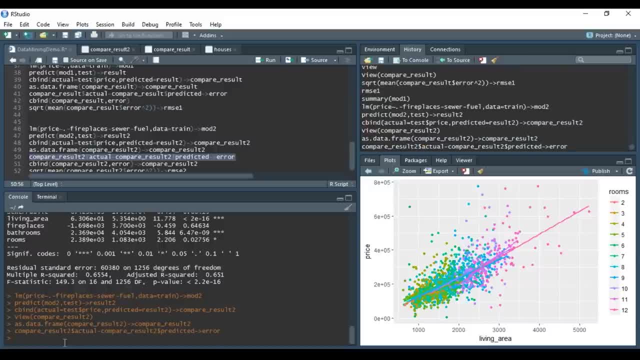 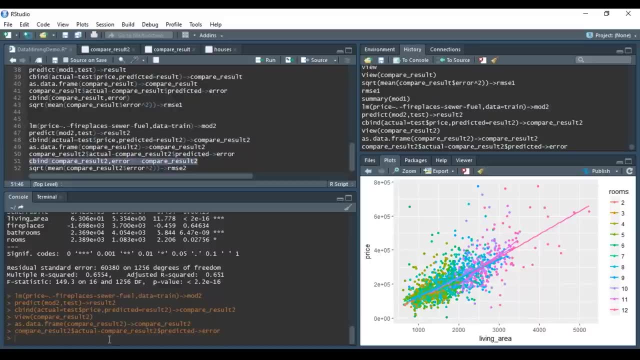 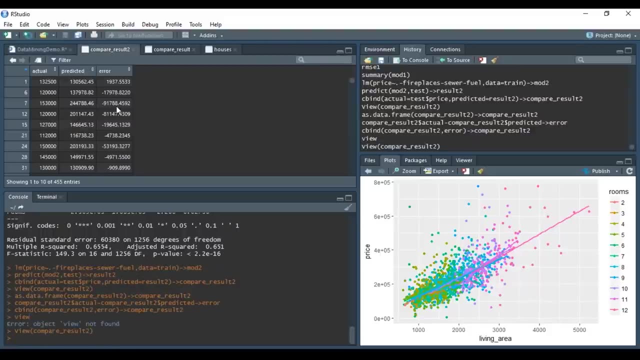 the error in prediction. So I've subtracted the predicted values from the actual values and store the result in error. Now also, let's combine the error in prediction to the same data frame set. Let's have a look at this: Actual values, predicted values and error in prediction. Let's go ahead and also. 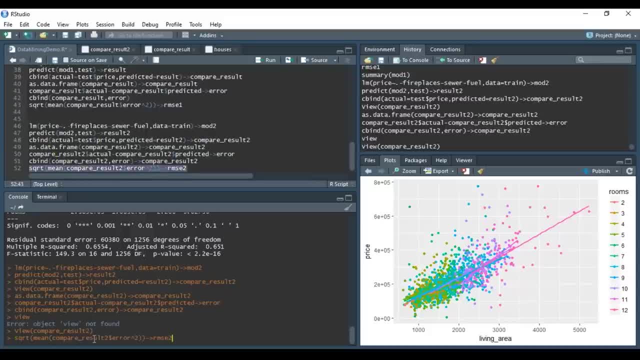 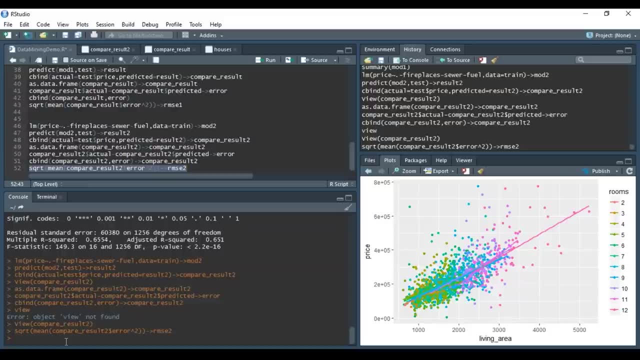 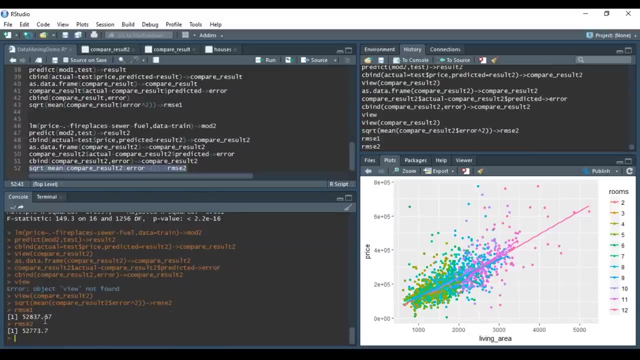 calculate the root mean square error of it. Root mean square error is simple, So we square the error and then we find out its mean and then we find out its square root. Let's compare the root mean square error of both the models built, So RMSE1. 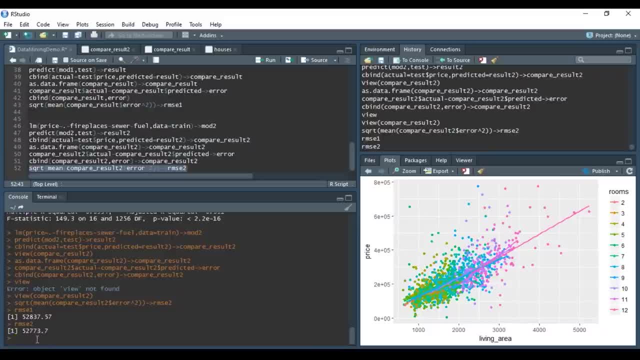 is 52,837.. RMSE2 is 52,773.. What we observe from this is the error of the second model is lesser than the error in the first model, and that is why the second model is better than the first model. Let's also have a look at its. 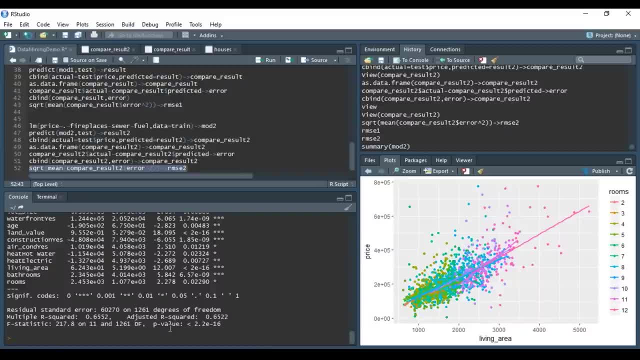 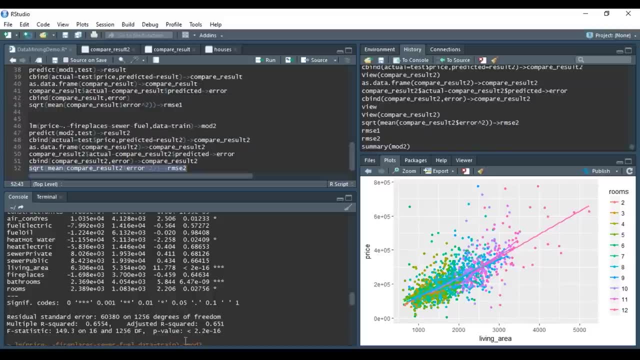 summary Summary of mod 2.. So its R-squared value is 0.6522 and the R-squared value of the first model was 0.651.. And since we see that this value is greater than the first model, again, so model 2 is better than the first model. 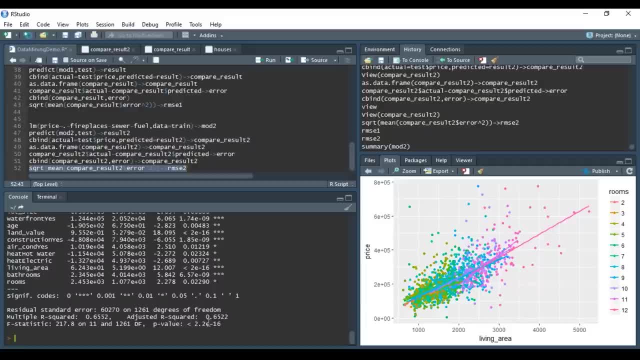 So this was it, guys, for the case study. We started off by importing the dataset with a bit of pre-processing, And then we used ggplot2package to visualize the correlation among the different data entities, And then we split the dataset. After splitting the dataset, we finally built the linear regression. 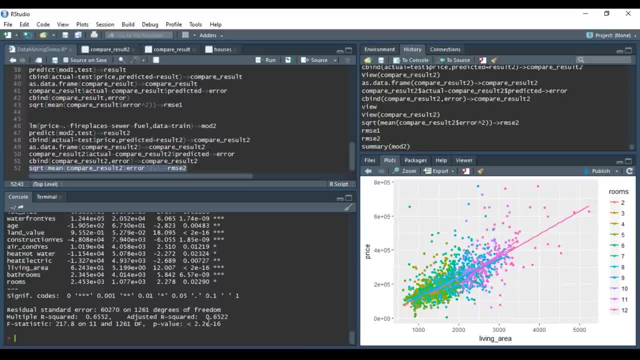 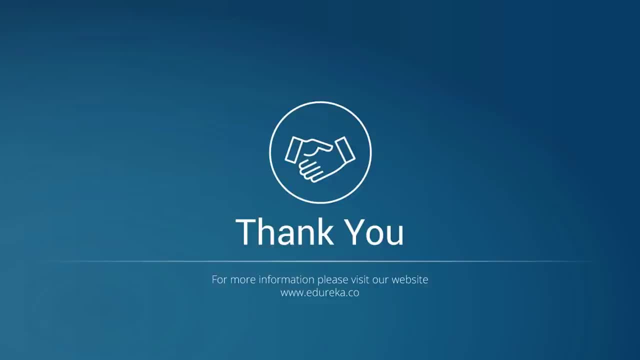 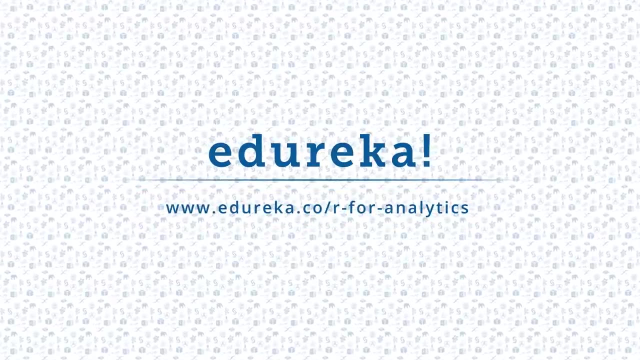 model. We actually built two models After that, But we have found out the accuracy of these two models and evaluate which performs better. Thank you for watching it. Hope you enjoyed it. Thank you, I hope you enjoyed listening to this video. Please be kind enough to like it and you can comment any of your doubts and queries, and.